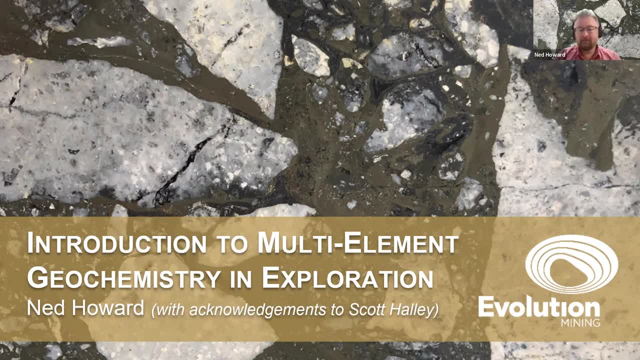 trying to show people how they can make the most use of all the elements you can get analysed for these days, But in a geological, geologically informed way, where you're putting that geological context on your interpretations. so yeah, and I'll acknowledge Scott Halley who's been a real proponent of this approach- 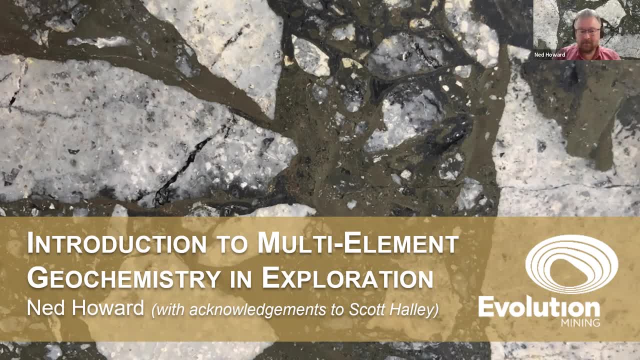 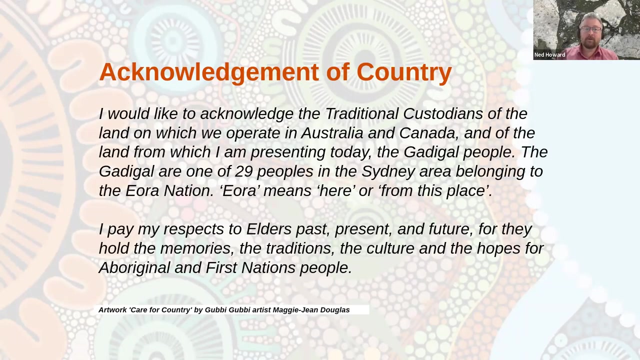 of using multi-element geochem and exploration for quite a long time now, and a number of you have probably probably heard of him, so I learned a lot of my stuff from him and he's got me my last two jobs. so yeah, big acknowledgements going out to him. I'd also like to give an acknowledgement. 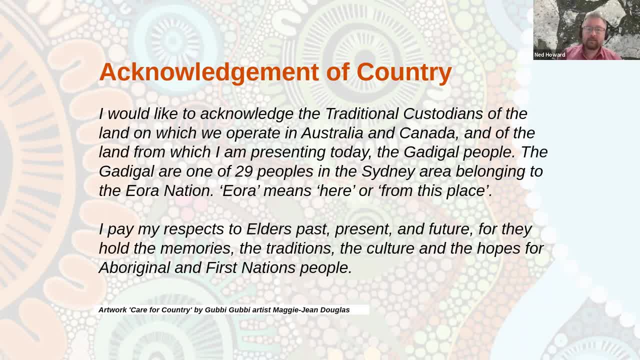 of country I'm presenting to you today, from Sydney, which is the home of the Gargoyle people, who are one of 29 different peoples who inhabit the Sydney area and belong to the Eora Nation. Eora meaning here or from this place. so I'll pay my. 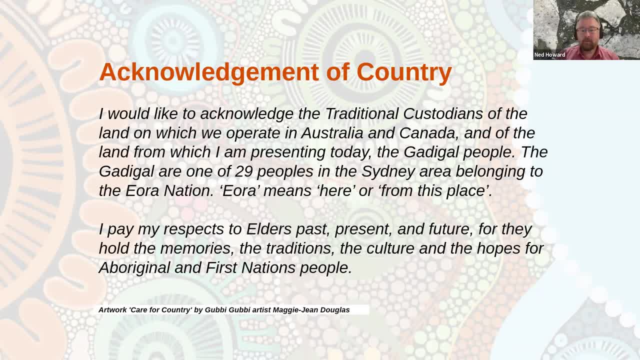 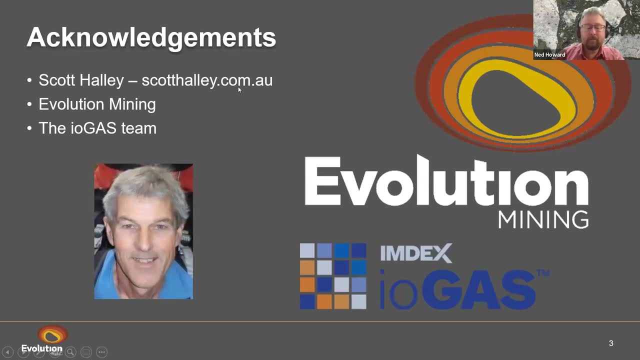 respects to elders, past, present and future, who hold the memories, the traditions and the cultures and the hope for Aboriginal and First Nations people here and right across the world, some other people to acknowledge there's. well, there's Scott Halley's web page address if you want to go and check out. he's got a whole bunch of presentations. 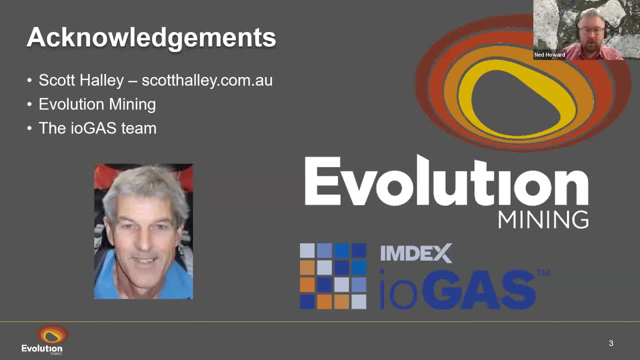 and other resources, tutorials and workflows for dealing with example data sets. so if you, if you're keen to follow up more, that's a that's a really great resource. I'd like to thank Evolution Mining, who I work for, for allowing me the time to to be able to undertake this. 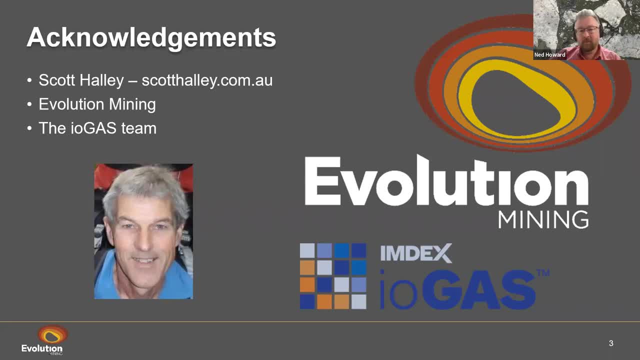 presentation and yeah, really is a great company to work for. I've really enjoyed my my time here. I've had some fantastic opportunities and got to work with a great bunch of people. and also- another acknowledgement: I'm going to be showing a lot of graphs from a program called iGAS, which a 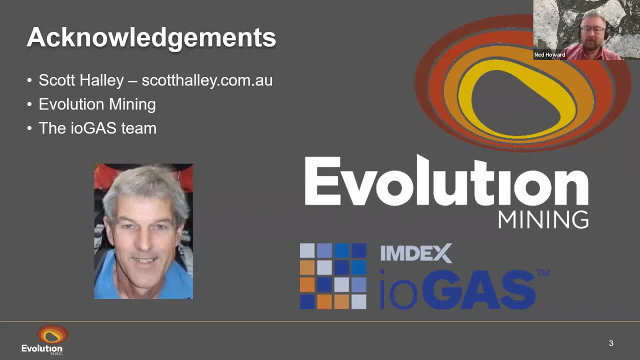 lot of you have probably heard of before, but this was originally developed by a company called iA Global, which has since been been brought out by by INDEX, but a lot of the key people are very much still there, all the same support and development people. and this is that, that software program in 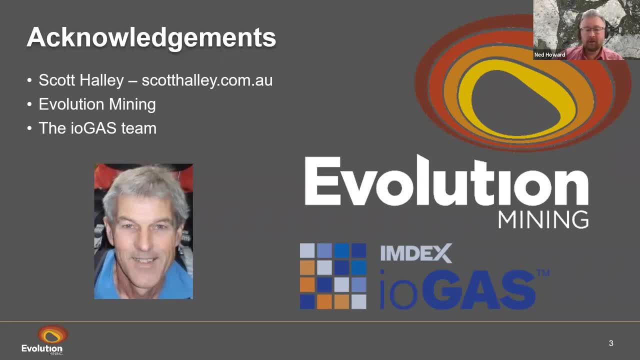 particular, has been kind of allowed a bit of a renaissance of the use of geochemistry in exploration, just for allowing people to to do things so much more easily and quickly and getting to know your data much better than than you really could before. so for an outline of what I'm going to talk through today, I've 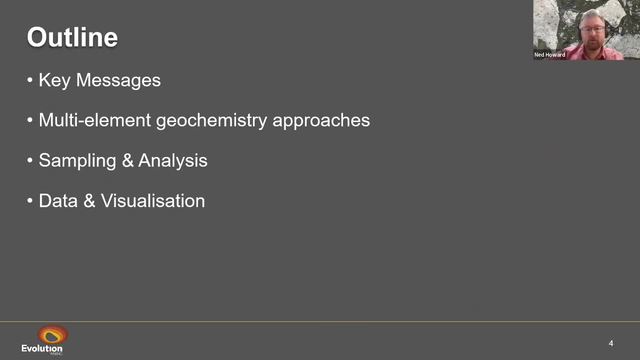 just got some, some quick key messages up front and then I'm going to talk through and give some examples, the different type of multi-element geochemical approaches you can use when you get full suite geochemistry. talk a bit about some considerations, with sampling and analysis not going to be able to cover, you know, everything, but just some. 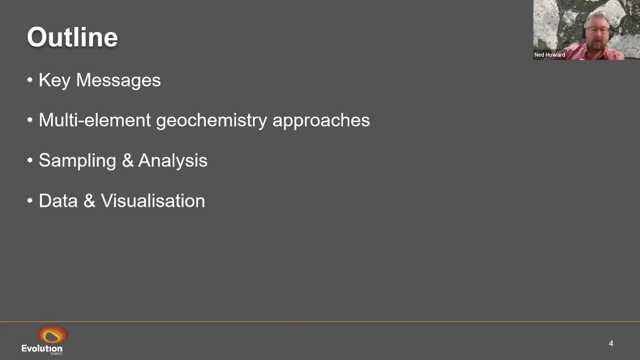 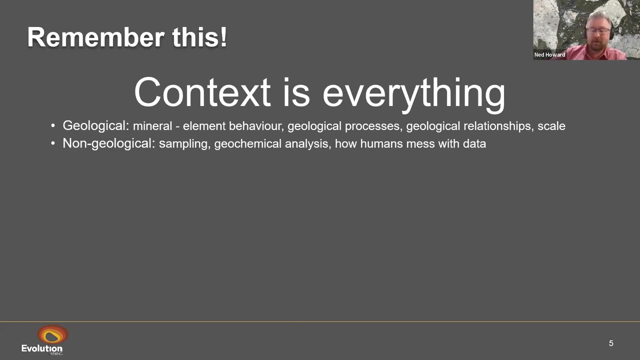 some, some key things that are that are really important to know, and a few notes on some aspects of data and visualization that either get on my goat or I think are really important. so first of all, remember, context is everything. I'm going to be talking about geochemical data. 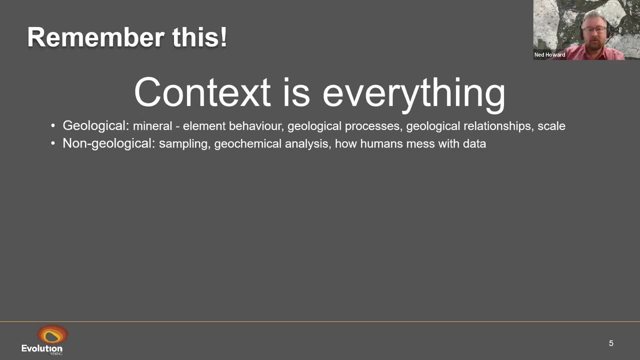 today. but it's super important to put that in geological context and that's about understanding mineral and element behavior, understanding and thinking in terms of geological processes, geological relationships, timing relationships, but also non-geological aspects. so you know how the sample is taken, aspects of the geochemical analysis and how. 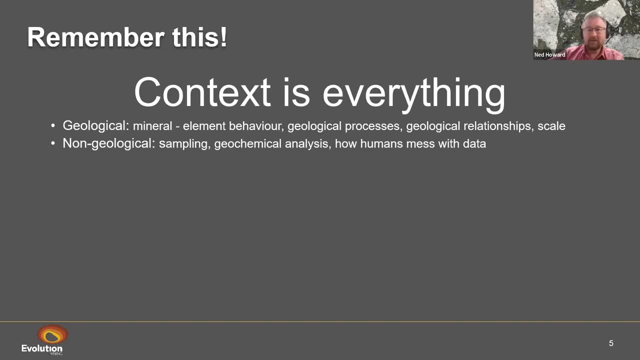 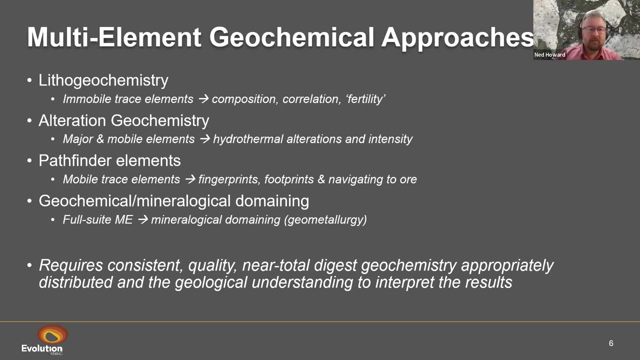 humans can really mess up with data, and geologists, in particular, are pretty good at this. so the multi-element geochem approaches that I'm going to talk about right now are the ones that I'm going to talk through lithogy chemistry, which is where we're. 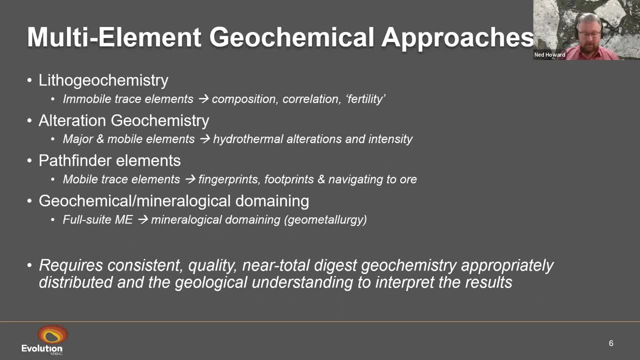 using a mobile trace elements, and when I say a mobile, I'm talking about elements that will not move around easily during hydrothermal or weathering related processes. so they hang around in the rocks and they're robust to those secondary processes. so where we're using those, 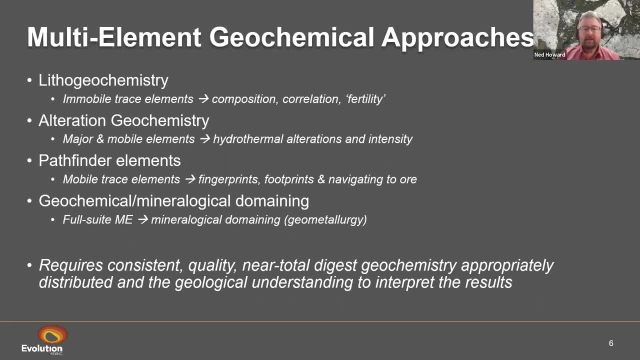 trace elements to classify and understand the differences in composition of the rocks we're looking at, so that we can then use that to be able to correlate different units, to recognise and separate out units that may look visually very similar or in terms of the major elements very similar. 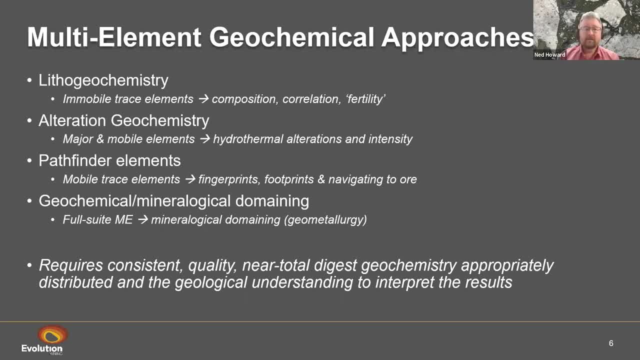 and also look at quote-unquote fertility indices, which is definitely a fad that we're going through. Alteration geochemistry, where we're looking at mages and mobile trace elements to understand hydrothermal alteration processes and map out the different types of alteration minerals. 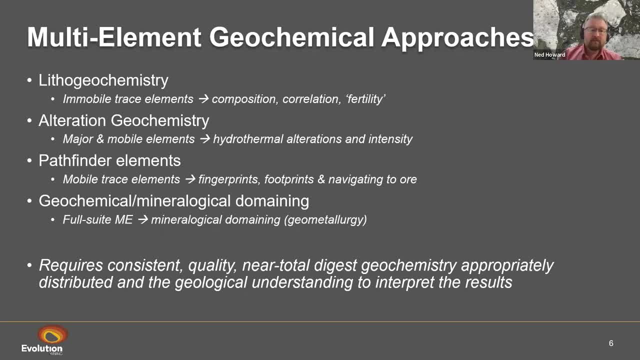 processes and their intensity, Pathfinder elements, so where we're looking at the concentrations of particular trace elements that are mobile and tend to form fingerprints or footprints around the rock. So there's a lot of information around gold or metal deposits, and understanding these can really help us navigate towards. 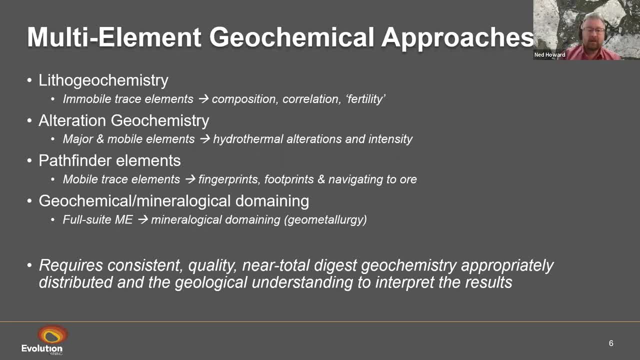 or help us understand where we might be in a system, And I'll mention just very briefly some application on geochemical or mineralogical domaining that can be really useful from a geometallurgy side of things, which is an increasingly popular topic these days as well. 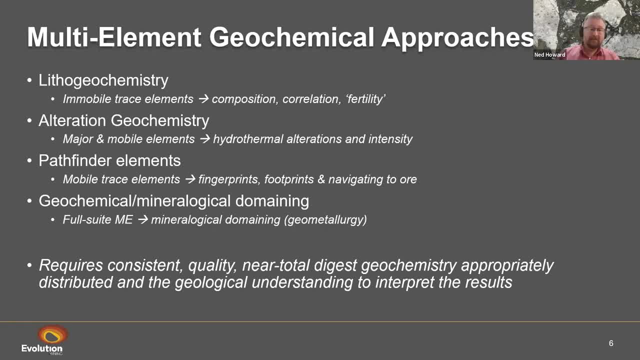 And I guess the next slide is just to show you, you know, just to note, there is that to you know, having consistent quality data, that's with a near total digest, like a four acid digest, and preferably analyzed with ICP-MS. 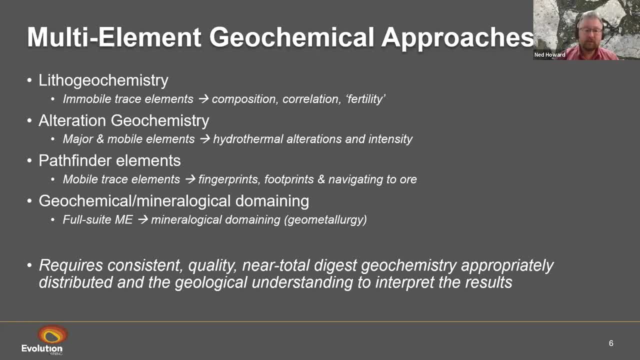 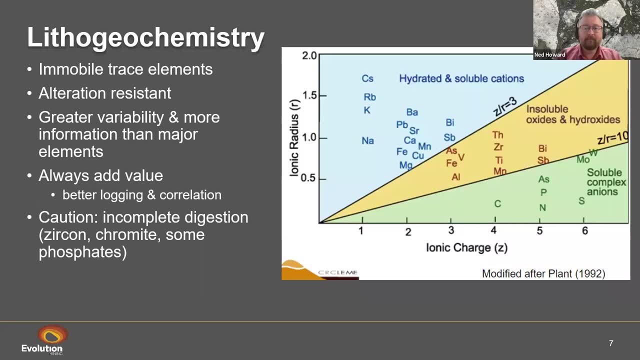 with a good distribution. appropriate sampling, sample spacing- is really important to being able to get the most out of out of any of these techniques. So sorry, I'm just going to move my screen a little bit, So to talk about lithogy chemistry, as I mentioned. 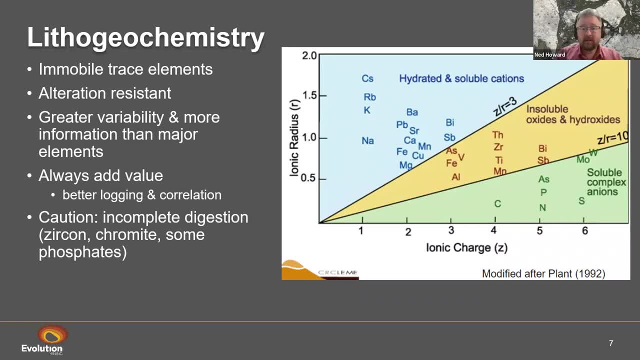 here we're talking about using immobile trace elements that are resistant to hydrothermal operation processes, So they're relatively insoluble in hydrothermal solutions or in groundwater during weathering processes. The reason why using these immobile trace elements is useful is because there's a lot more of them. 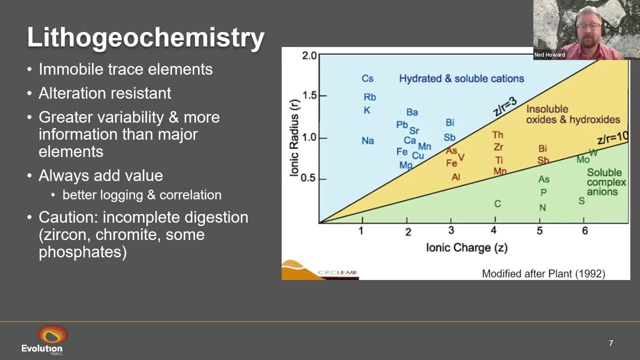 and they show a greater variability in how they behave than the major elements. So we're actually able to pick differences out and discriminate different rock types on the basis of their trace element geochemistry. that we just wouldn't be able to do with our major element geochemistry. 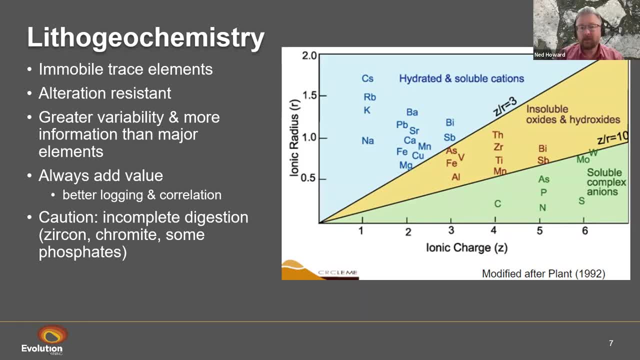 Not to mention that most of the major elements are also relatively mobile and move around a lot during those secondary processes. So I've never had a circumstance where lithogy chem hasn't added value Again. you always want to integrate it with your geological logging and your other data sets. 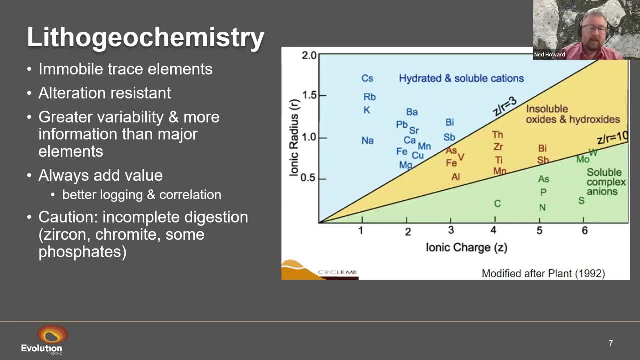 to get the most out of it, but it always helps. So this image over here- I'll just put my laser pointer on- is showing what are the key controls that determines how elements behave and the patterns that they behave in. So this image over here- I'll just put my laser pointer on. 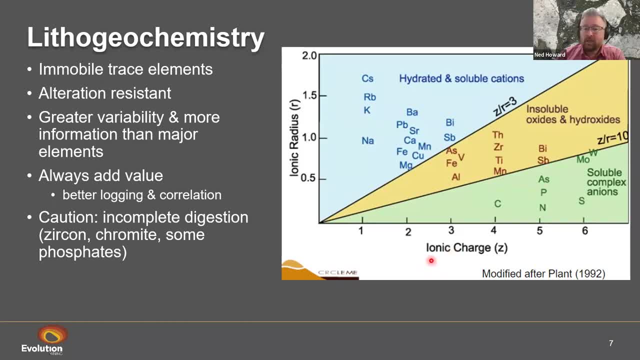 is showing what are the key controls that determines how elements behave in those. So here we're looking at the ionic charge of an ion versus the ionic radius, And so we'll see things that are clustering on this graph are things that will tend to behave similarly. 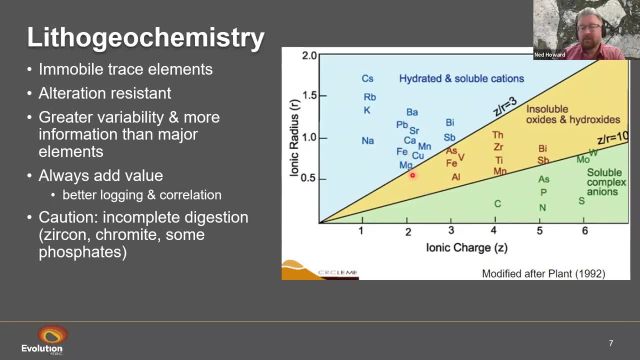 And usually what that means. you're looking at where the major elements are sitting, and then the trace elements that have a similar ionic radius, ionic charge will usually behave similarly and tend to substitute into the minerals that those major elements will go into. 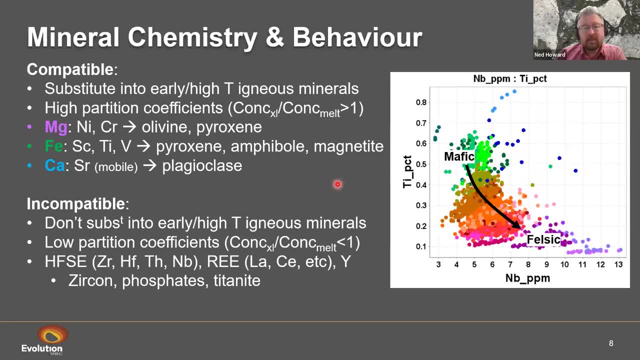 So mineral chemistry and behaviour, Usually here you know. so we're talking about looking at a couple of different types of elements, those that are compatible and incompatible, And usually when we're doing a lithogeochemical discrimination plot, we'll plot one of these against the other. 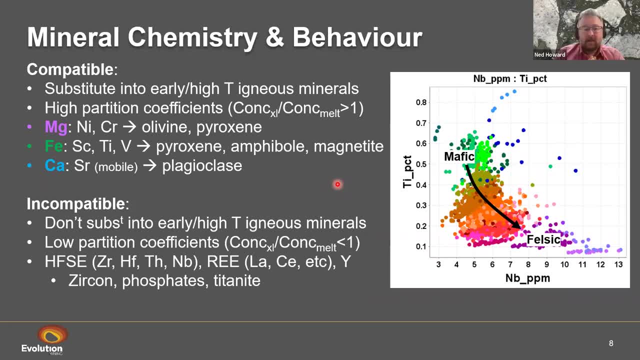 But what I'm talking about with compatibility here is the propensity of elements to go into a particular mineral that's forming, And so understanding lithogeochemistry and being able to interpret the patterns that you see, it's really important to have a bit of a context. 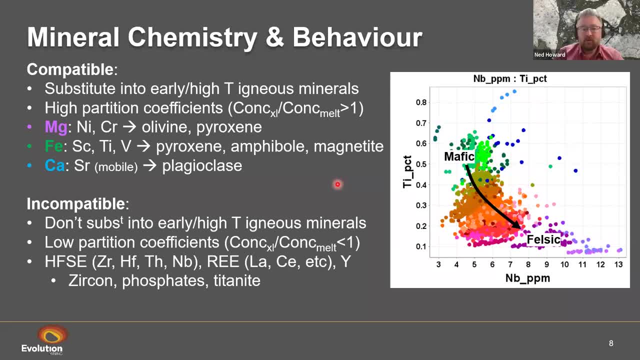 for the kind of minerals that are forming during geological processes And how, and the behaviour of particular elements with respect to those minerals that are forming or dissolving during geological processes. So compatible elements are elements that tend to substitute into early, usually early formed. 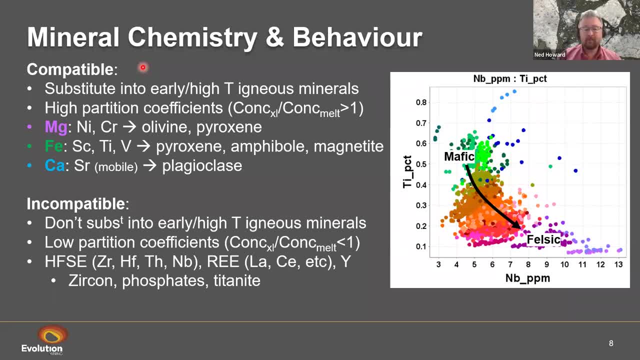 and higher temperature formed minerals. If we're talking about igneous fractionation, which is often, you know, usually we're often where we're dealing in environments that are where we have a lot of igneous rocks, whether they're volcanic or intrusive. 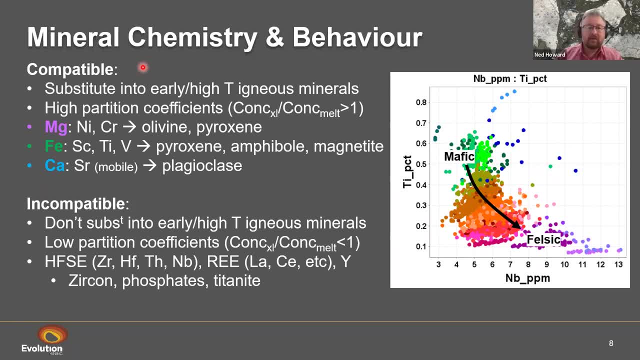 And so these igneous fractionation processes are a really important part of putting of understanding what's going on with the composition of our rock. So with compatible elements are those that tend to substitute into early formed and high temperature minerals, which means they have high partition coefficients. 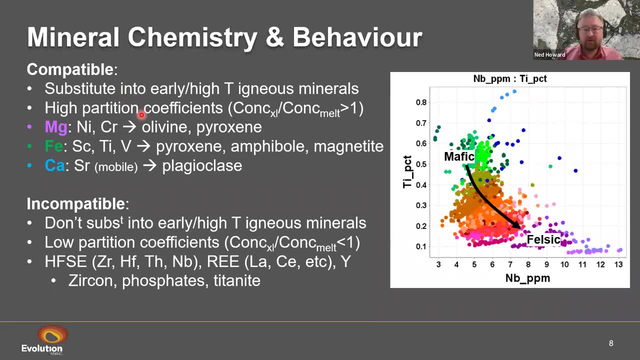 So they tend to. they'll have a higher concentration in crystals that are forming early over the concentration that's remaining in the melt, And we can think about this in terms of associations with different elements, So those trace elements that tend to follow magnesium around things like nickel and chromium. 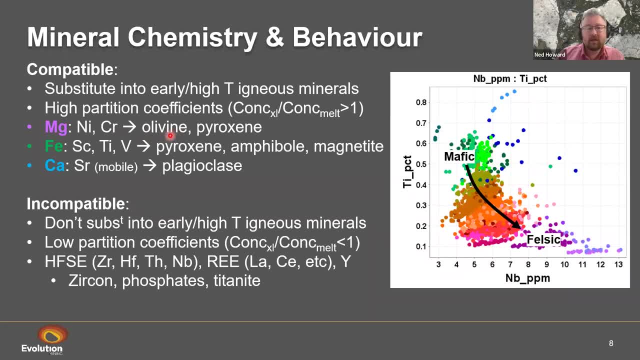 And so they will generally substitute preferentially into crystals like olivine. minerals like olivine and peroxine Trace elements that have an affinity for iron and fairly serophile are things like scandium, titanium and vanadium. So they'll follow iron into minerals like peroxine. 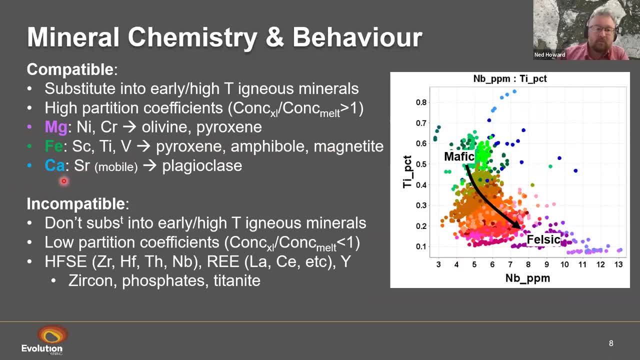 amphibole and magnetite, And then strontium, though that is mobile, will tend to go into plagioclates. Some incompatible elements are ones that tend to hang around in a melt and don't go into those early formed minerals. 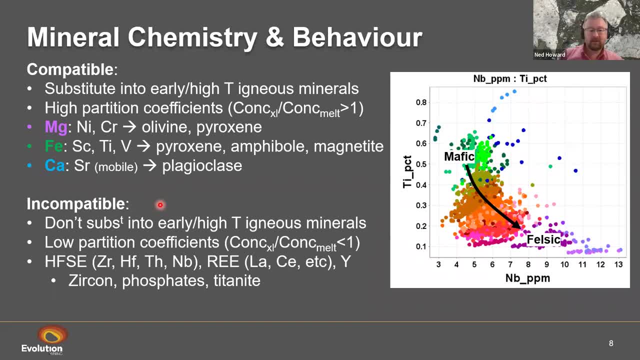 So they will tend to increase in concentration through the fractionation- igneous fractionation- process. So what we're talking about here is some really useful ones to use- are the high field strength elements, So things like zircon, thorium and niobium. 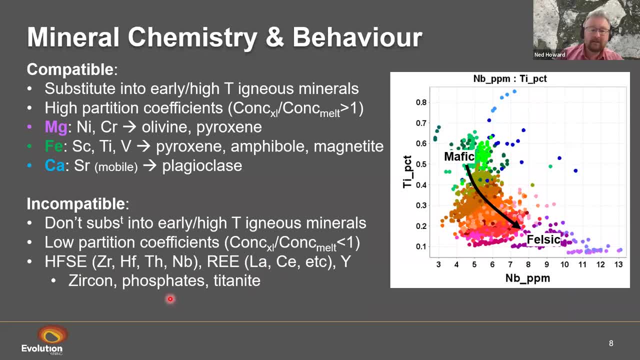 also rare earth elements. These tend to go into later forms, phases, resistate phases, like zircons, phosphates and potassium. They can also go into some of the molybdenum-type molybdenum. So usually what we'll see with the patterns that we see. 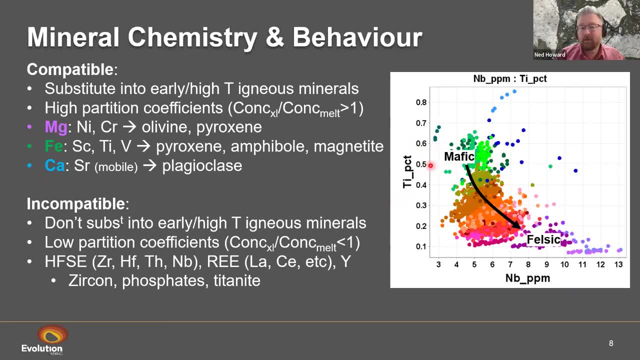 in this kind of data from rocks. if we're plotting a compatible element up here on our y-axis and then an incompatible element on our x-axis, we'll go from relatively high concentrations of things like titanium and other compatible elements down to, and as we drop in, the concentration of those elements. 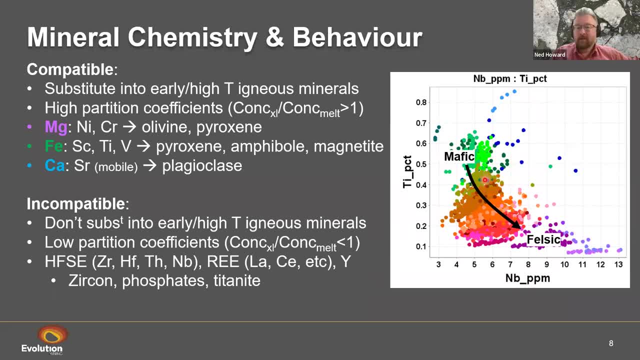 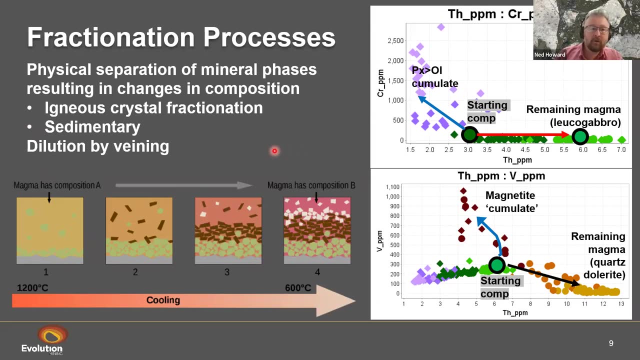 tend to increase in concentration of the more incompatible elements. So usually, you know, one of the best ways to split out the differences that you're seeing in the composition of your rock units is putting these against each other. So fractionation processes I've already mentioned. 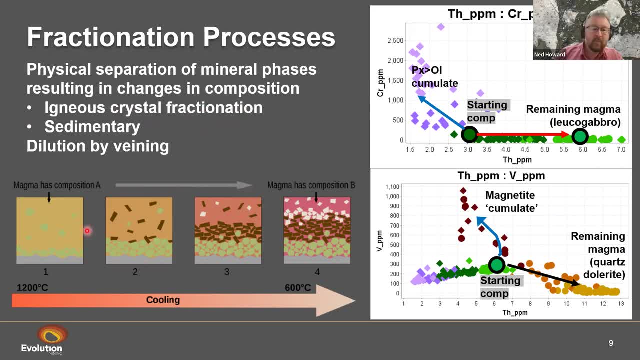 the importance of igneous crystal fractionation, but just to touch on that a bit more. what we're talking about here is when we have a magma and it starts to cool in some kind of lower or some lower below crustal or crustal magma chamber. we'll start forming these minerals like 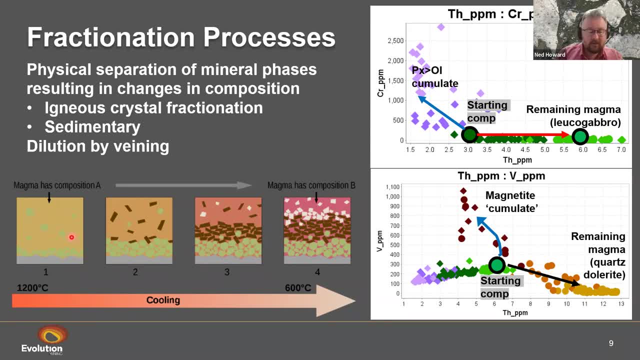 olivine or peroxine, and usually they're denser than the melt and they will start sinking down into and accumulating at the base of those magma chambers. So the thing is this: is these minerals, and they're going to start sinking down into and accumulating at the base of those magma chambers. So the thing is these minerals. 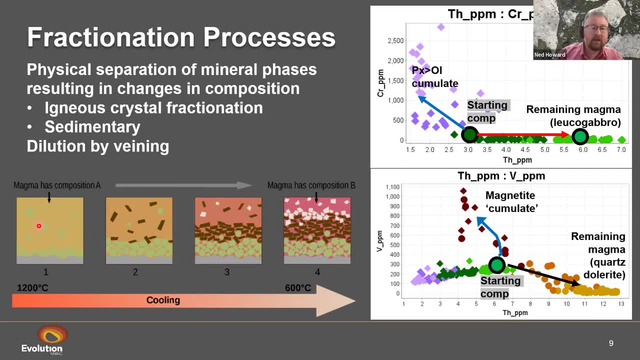 will suck up trace elements at a greater rate than some other trace elements. So if this was olivine or peroxine, we'd expect a lot of our nickel and chromium to go into these minerals and that will deplete the remaining melt in those elements and then it will concentrate them. 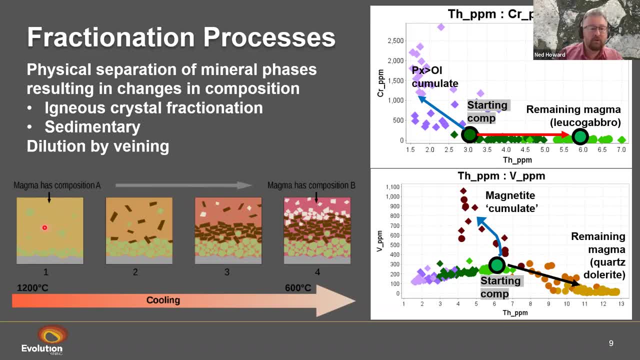 at the base. So firstly we have minerals preferentially going into sorry elements preferentially going into minerals, and then they're being physically separated from the rest of the melt That can then move away or has change in net composition. So we might get that happening initially with some olivines, or we might have peroxine or 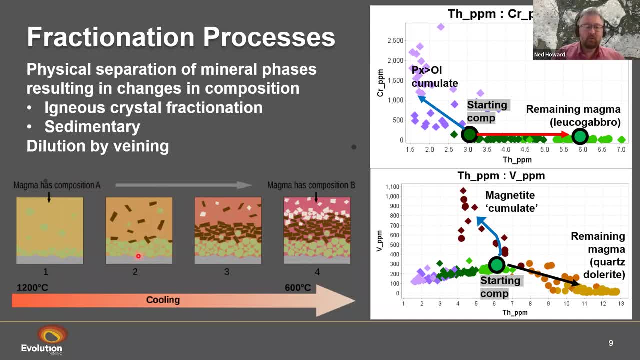 hornblende doing that and then some other later, formed mineral and will gradually change the composition of the melt as we go through that process. We can also see other fractionation processes. They can be mechanical processes during in within epiclastic sediments. We can also see things like dilution by veining in our samples. 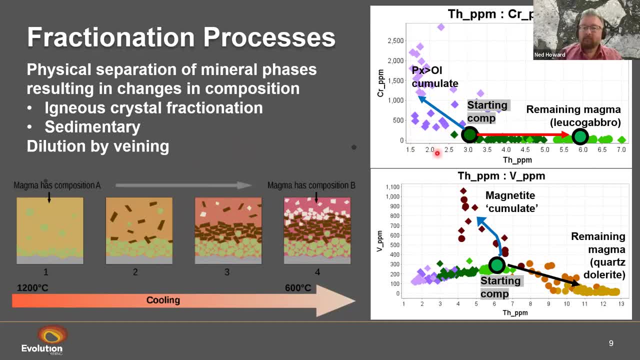 if you've got a lot of veining in them. So one example of what that looks like in the geochemistry is an example from a fractionated dolerite seal in the eastern goldfields. So we might have a starting composition in that magma around here and as that starts to crystallize, 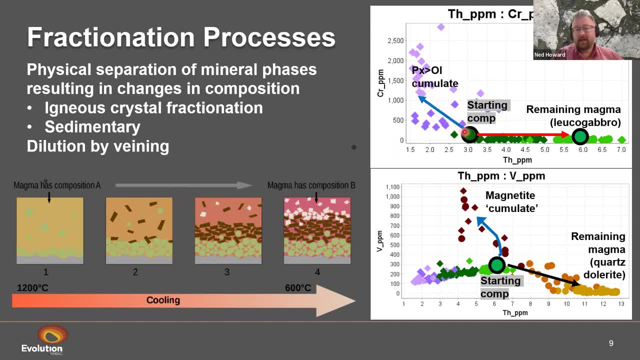 we can see that the, the, will be gradually more and more concentrated within the remaining melt, So we'll change the overall composition of the magma to maybe a leukogabril after some time that. what you might then get is that a change in the, the mineral that starts fractionating. 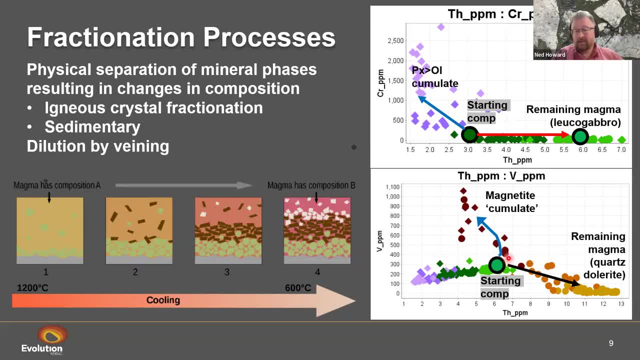 and we, we start producing magnetite that then settles out and separates from the melt as well. and so what? we'll see? that that magnetite cumulate will have really quite much higher concentrations of things like vanadium and titanium, and the remaining melt will be relatively depleted. 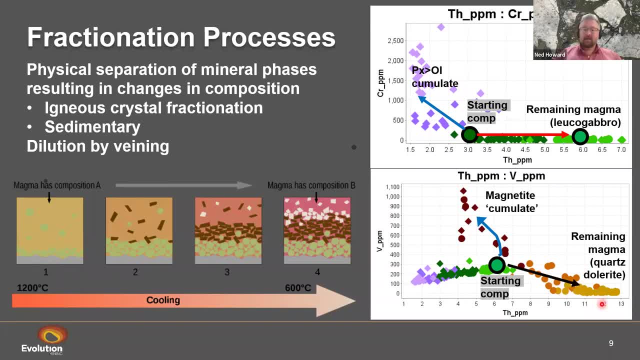 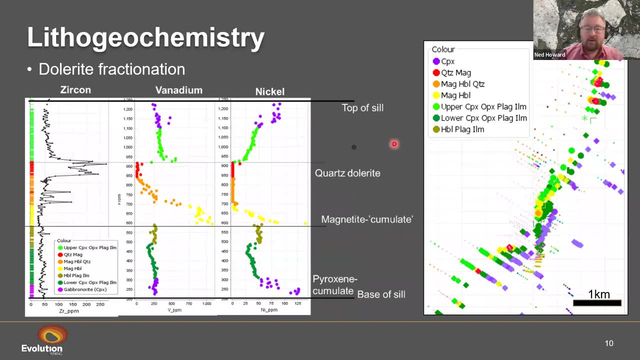 uh in vanadium and continue to to increase in um in thorium and zircon and elements like that. so how we can see that that fractionation process in a a bit of a microcosm is like. this is a downhole plot. so those different elements, so you can see um, the, the um. 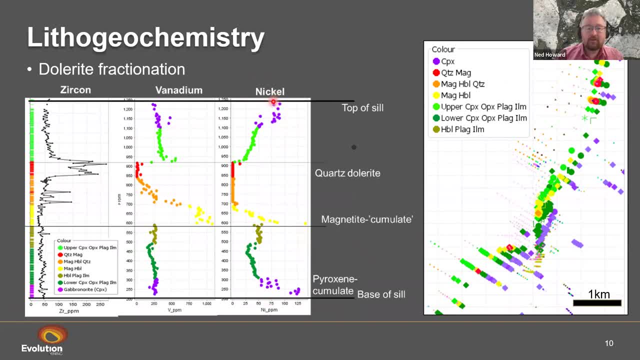 the, the bulk composition, usually right near, near the, the top contact of the seal, um, where we're seeing um, uh magma that's been frozen before it's, it's had a chance um to fractionate um, and then we'll see these cumulate zones where we've got relatively high. 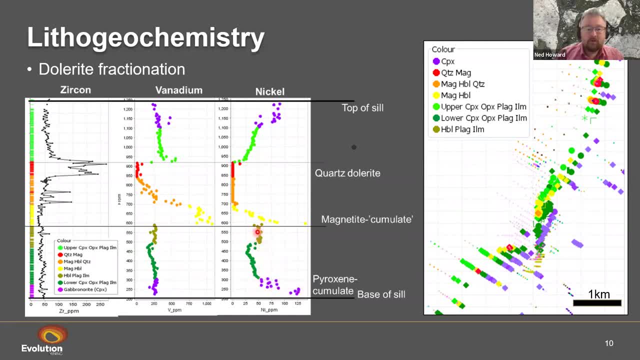 nickel and chromium and things down the bottom um. as we move up through a seal and start getting magnetite fractionation um, we'll get really high vanadium um and uh, and then the the resist. the remaining melts from that will be strongly depleted in things like vanadium um, but we'll see. 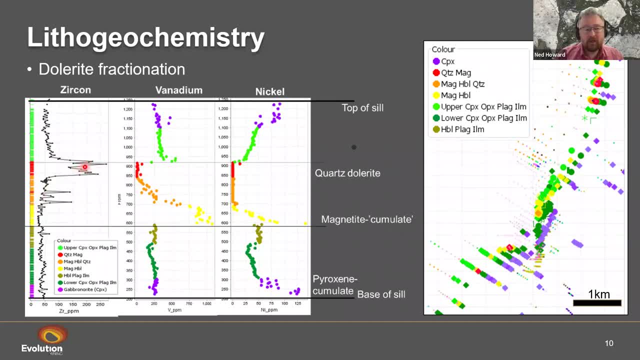 a gradual increase in the concentration of the mode of uh incompatible elements like zircon, uh in in those, those last fractionates within those seals, and so you can then plot that out, um, and map out uh, essentially the internal stratigraphy within those seals and areas where you might be getting better development of of the final quartz. 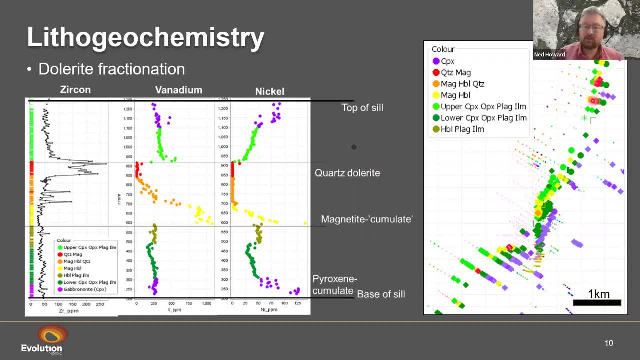 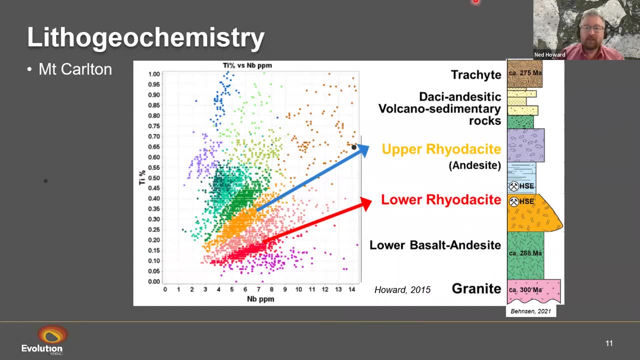 magnetite, um dollarite- the graniferic dollarite, which is usually the last phase, and um is- is often a preferred host rock for gold deposits in the eastern gold fields. one of the other things, one of the reasons we want to do with the geochemistry that's really. 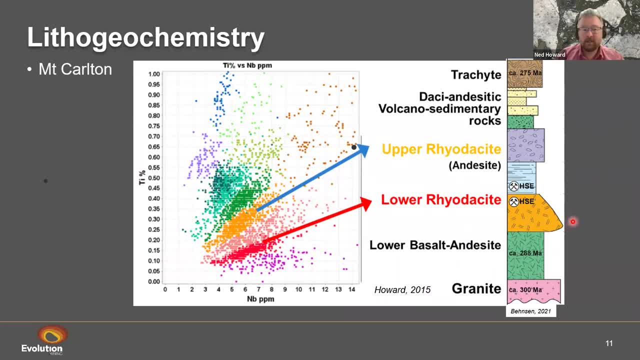 useful is that it can allow you to discriminate rocks that otherwise look very similar to each other. this is an example from the mount carlton high sulfidation epithel deposit in queensland and where, um there, we see some, uh, quite broadly developed and very intense. 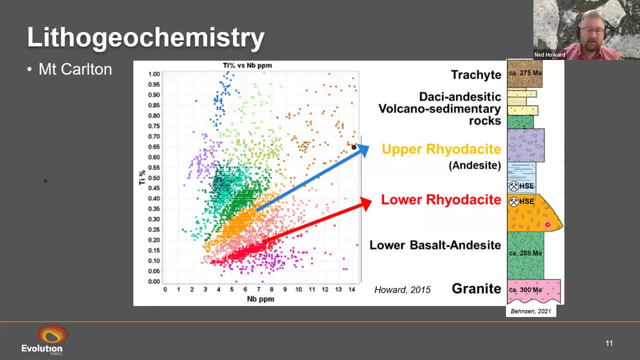 hydrothermal alteration that basically blitzes the rock so that um once it's been altered, um by advanced argillic alteration, usually it's just a mixture of quartz and clay. um we can't. it's very hard to differentiate what it is um, so we went in there when um i first joined, um evolution. 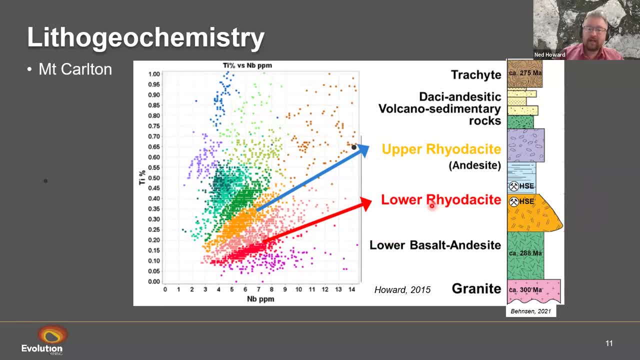 and did some lithogy chemistry and differentiated out two different rye day site horizons that were advanced, argillic altered but in in some places these had not been differentiated properly and in places you know drilling had drilled through stratigraphy and tested this top rye day. 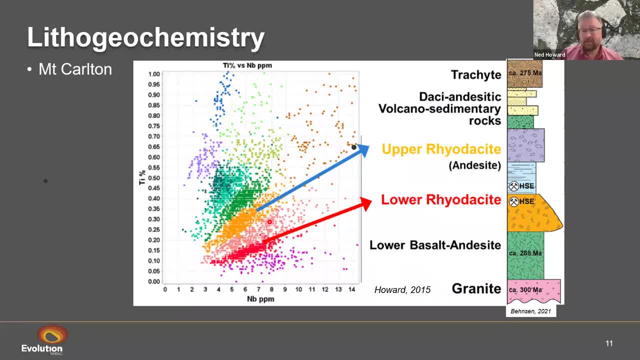 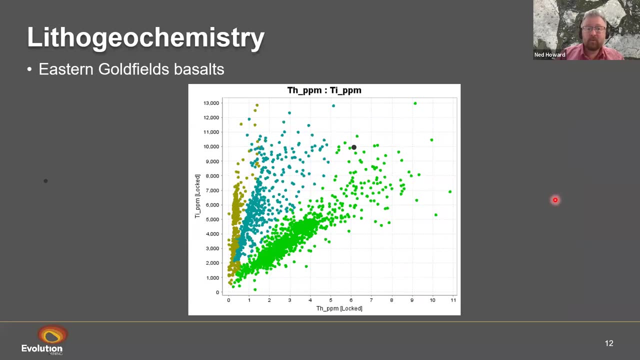 site, but then the whole had been stopped because they thought they tested the, the main ore hosting horizon. when it was done, actually the the lower rye day site was was still down there by where they drilled the hole to in the eastern gold fields. you know an example of of where we can differentiate out otherwise. 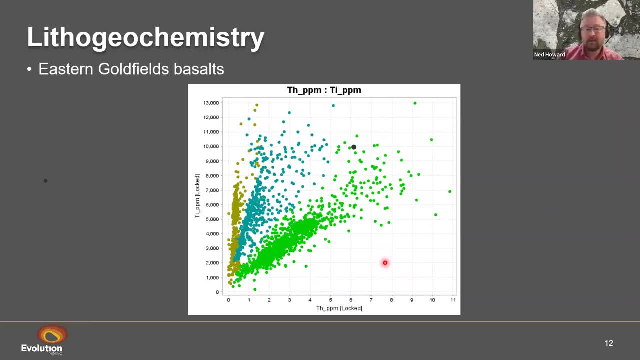 very similar looking rocks is with different types of basalts. so this is an example from from our mangari project. these are all basalt samples, but on the basis of the titanium thorium ratio you can pick out these, these different types that sit at different positions within the stratigraphy. 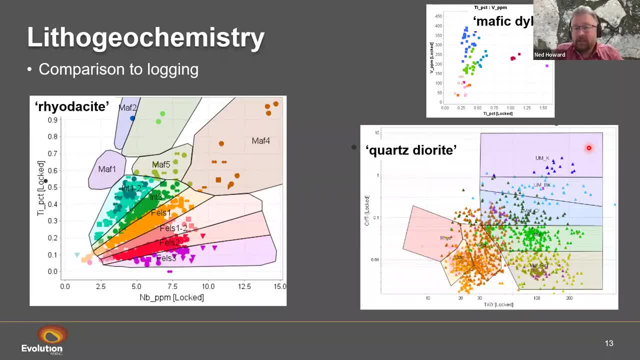 so, in comparing that to logging, um, obviously you know, logging is a absolutely critical part of it and there's things you can see visually in a rock that you might not be able to see in the geochemistry but often in the geochem. uh, we've got a data set that's relatively more objective in some ways and can 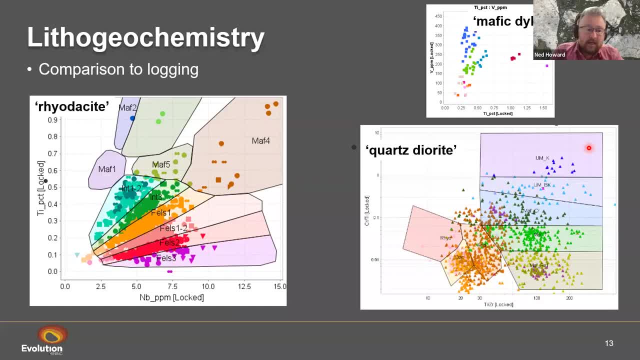 allow you to get a much more consistent um classification of the rock type than you might get with relatively inexperienced or varying geologists. uh and dealing with a range of of altered and and and weathered samples. so this is an example here again from the mount carlton project. 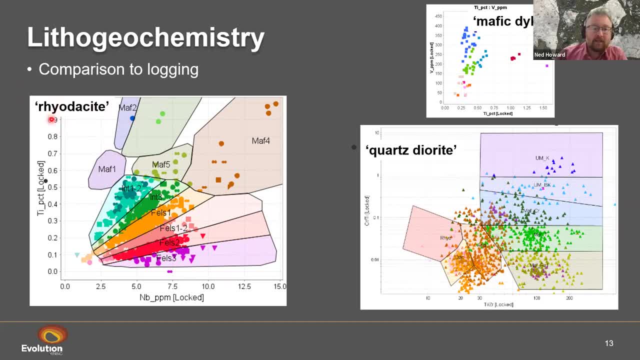 where all of these samples here have been logged as a rye day site because they're all smashed with with hydrothermal oil duration. but actually what we're seeing in in rocks that have been logged as rye day site is the full spectrum um, right from genuine briar day site through to intermediate and mafic rocks. it's just that. 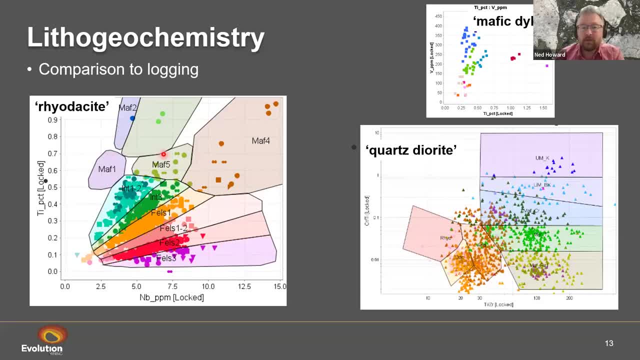 they've been been really strongly altered to the point where the geologist couldn't tell the difference. um, here's another example from a different deposit. all of these samples have been logged as quartz diorite, but we're seeing things right through from from ultramafex to fractionated 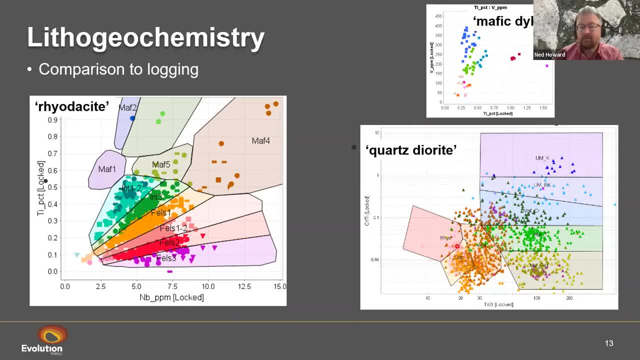 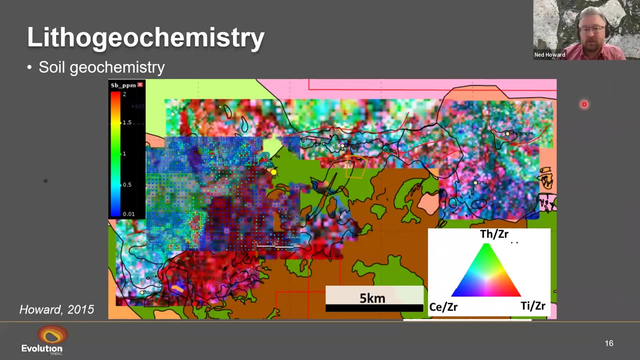 iron tholeites to andesites and dacitic composition materials and a similar thing here with what have been logged as mafic dikes showing a full compositional range. another thing that you can do with lithogy chemistry is is apply it to soils as well, not just to rock. chip samples, um, and where you've got, you know. 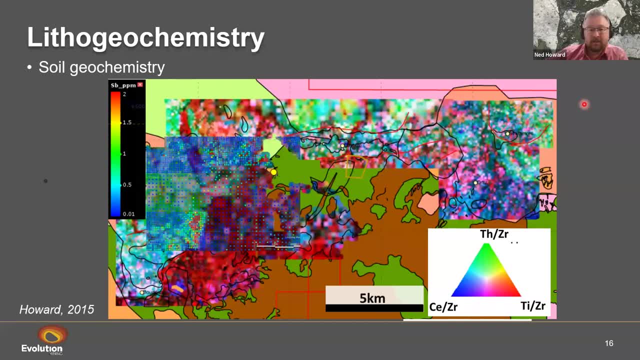 residual soils. you can usually create a pretty decent geology map or assist you in in building your geology map so that you can see what's going on in the soil. so this is is one example where i've made a ternary image um of titanium to cesium to thorium- through here and you can see that it's mapping out. 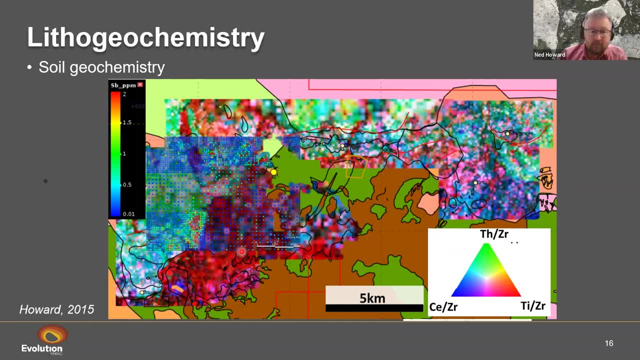 some different geology through here quite nicely and in particular, you know we can see this quite prominent boundary between the more mafic titanium rich red group through here, um, and we're seeing in this area where we've got um antimony soil sampling, you can see that the anomaly there is being truncated quite clearly. 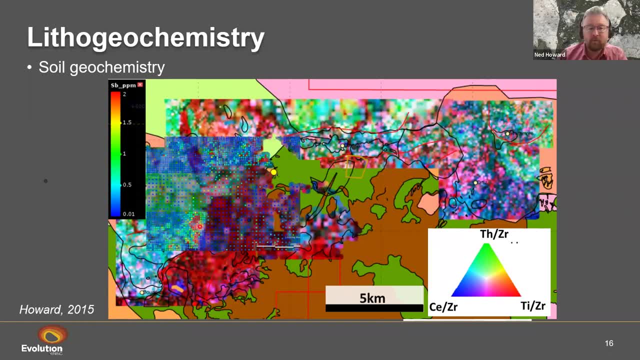 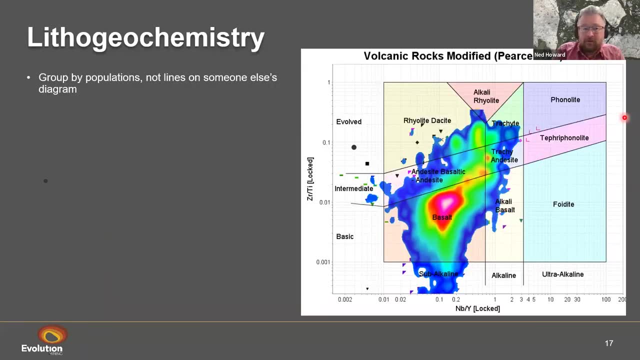 by that boundary. so that's, that's an unconformity, that's defining pre and post mineral rocks, a couple of to do's or don't do's with lithogy chemistry. you often see a lot of people and they'll try and classify things on the basis of of published rock classification diagrams. 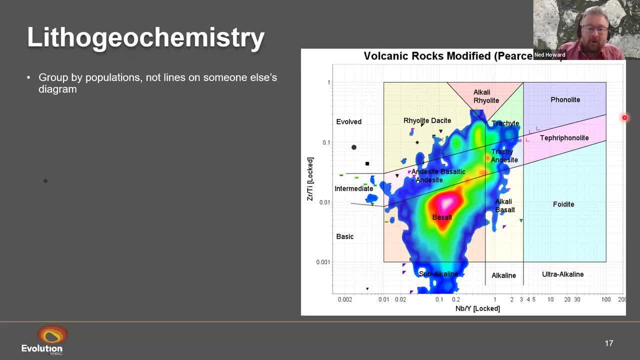 um, i don't recommend you do this. um often they were built with specific purposes that aren't necessarily appropriate to your data set or the composition of rocks that you're seeing and also you know, something that people will often tend to do is is cut groups and define groups on. 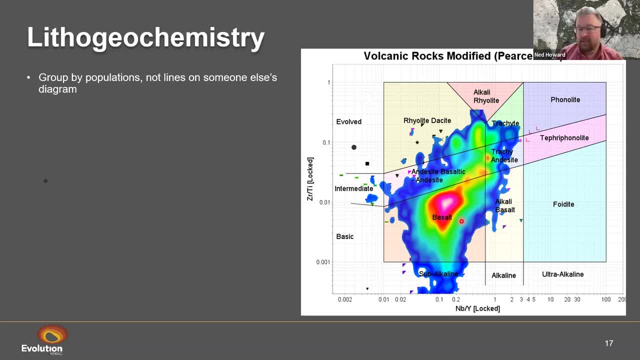 the basis of those, those hard lines, when you can see here, um, on this, uh, on this point, density contour, here on this, uh, on this point density contour that we're actually, if we, if we cut, we're actually if we, we cut these rock groups along these lines, firstly, we'd be including things from that group and that. 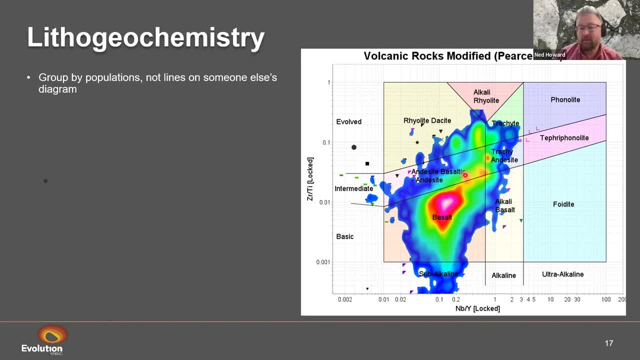 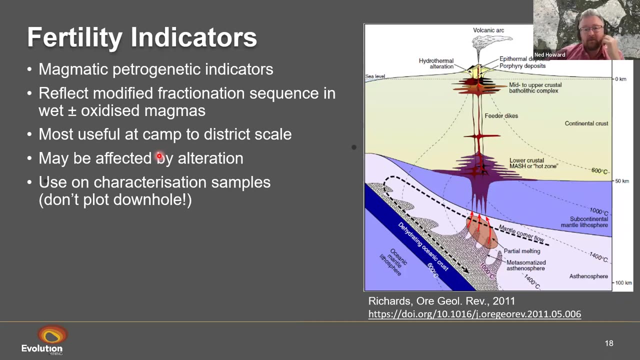 group in the same thing, which are different populations, and also we'd be cutting those two populations in half. So classify on the basis of populations within your data, not on the basis of lines on someone else's classification diagram. The other thing we can do with multi-element. 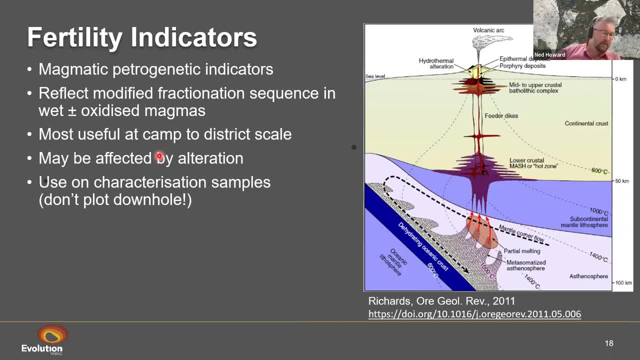 geochemistry is: look at fertility indicators. So usually what we mean by this it's usually around igneous rocks, around intrusive rocks that are thought to be genetically related to and spatially associated with mineral deposits of some type. So the classic one here is porphyry. 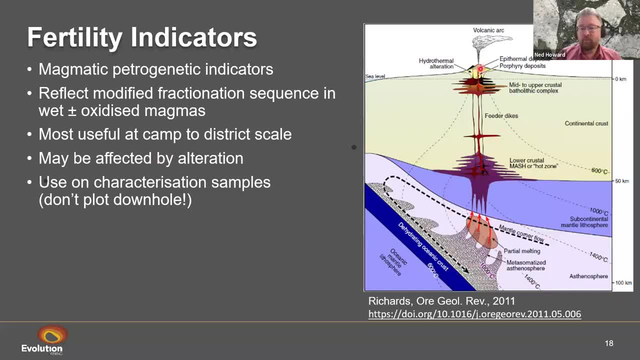 deposits. So we're seeing a cross-section showing the overall processes that are involved in producing some porphyry, copper plus minus gold or moly deposits, and all the processes that are involved in changing and getting the composition of the magmas to be able to release a hydrothermal fluid and produce that deposit. 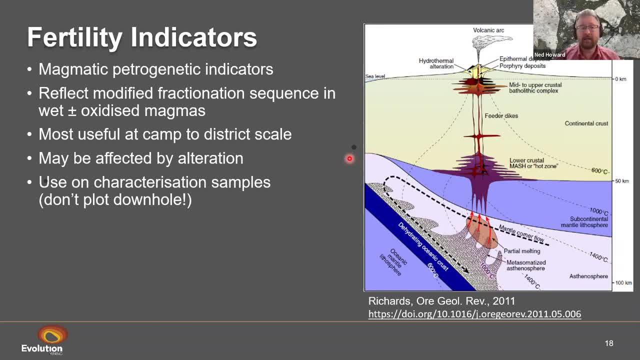 So usually these, what we're looking for here, are geochemical indicators, within in the chemistry of intrusions that are reflecting the formation or not of particular minerals that reflect some important characteristic of the magma, and usually that's to do with what we're trying to detect is where magmas have been wet, and usually where they've been in the case of porphyries, where 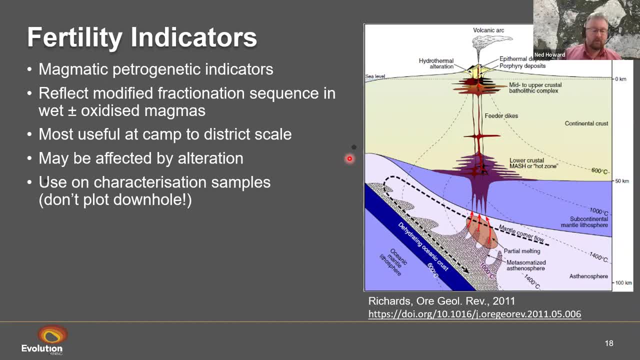 they've been relatively oxidized. It will depend on the metal and the type of thing you're looking for, but like almost all intrusion related deposits, you want to see indications that a magma has been wet and that's affected the crystallization order of minerals. that then has an impact on the chemistry of the resultant magma that you see. 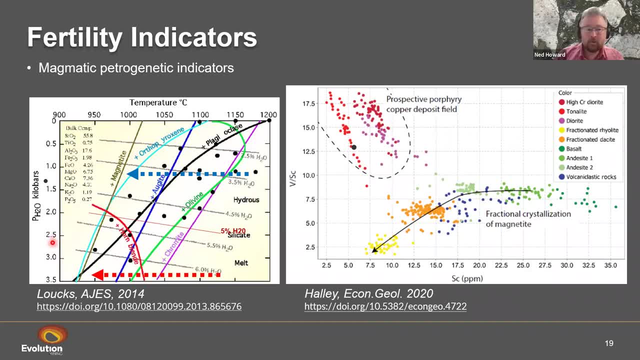 So for an example of that here, here is what might look like a quite a complicated diagram, but what it's basically showing us is that, as a function of the pressure of water- so essentially the water content and temperature, what minerals we would expect to be seeing? 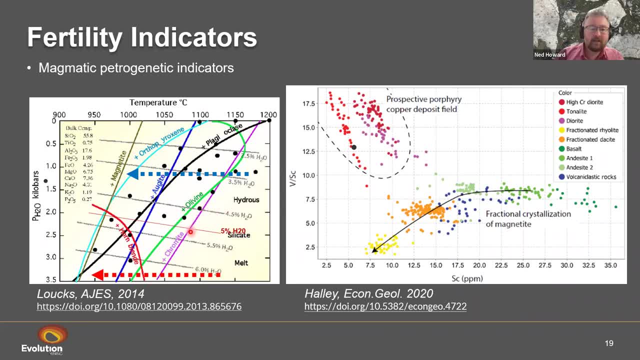 So if we start with a melt out over this side and then these lines define when you will start, as you cool, so you go from right to left, what when you would start expecting to see those minerals forming? So if we had a magma that was relatively low in water, so about, you know, three percent or so? 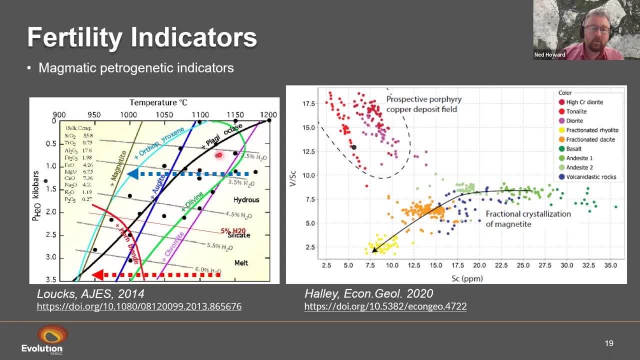 as we cooled that magma, we would expect to see plagioclase and peroxin forming before we start seeing magma, and we're probably not going to see hornblende forming, Whereas if we see, if we have a magma that's rallied and we start to see what's causing aimitta and Ee, and we're probably not going to see hornblende forming. 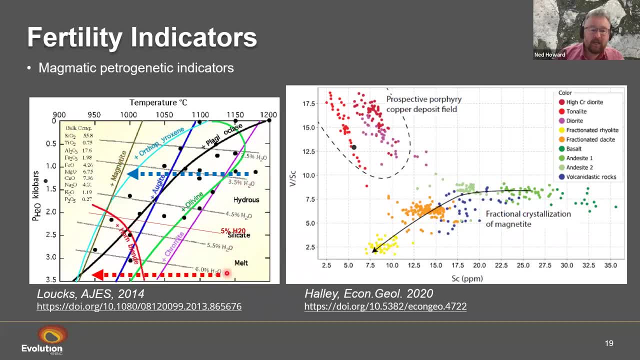 slash 圴, whereas if we see, if we have a magma- magma that's quite high in water, so it has, you know, six percent or so water- we're going to see quite a different fractionation sequence and, in particular, we're going to start seeing horn blend. 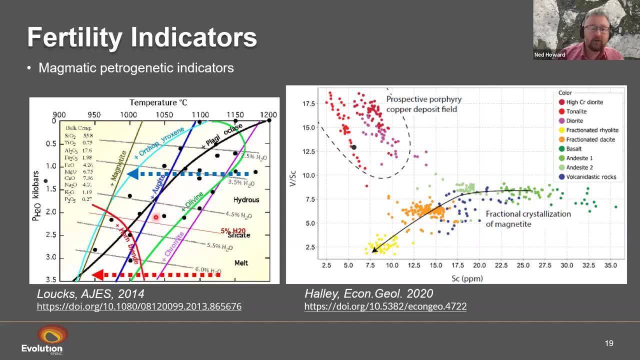 we'll start crystallizing before we get either, you know, olivine or or peroxine or plagioclase, and we're also going to see horn blend before we get to to magnetite as well, and so what we get what we then see with that is that by having horn blend fractionate early, we will pull out our 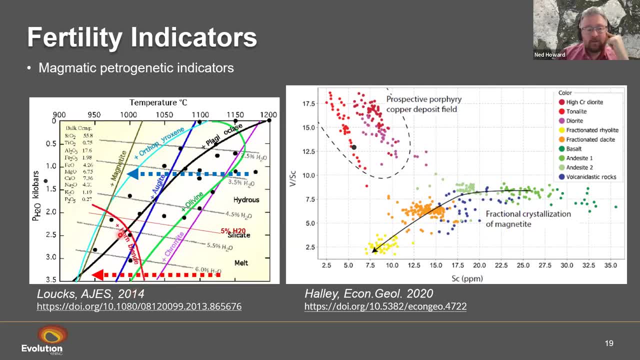 scandium out of the melt. but because we're doing that before magnetite, we're going to continue to let vanadium build up in the melt, because vanadium would go preferentially into magnetite and get depleted in the melt normally if we had magnetite fractionation. so it's really picking that. 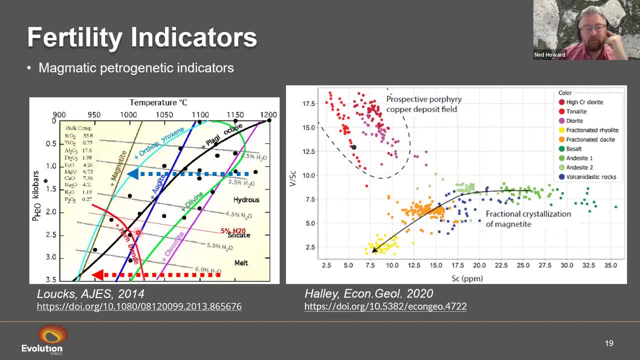 difference between where we're getting magnetite coming in before or after hornblende, and so that's what this diagram is showing. here is the example from scott again. so with magnetite fractionation as we decrease in in scandium, as we're getting more and more fractionated, more felsic, we would see the vanadium over scandium. 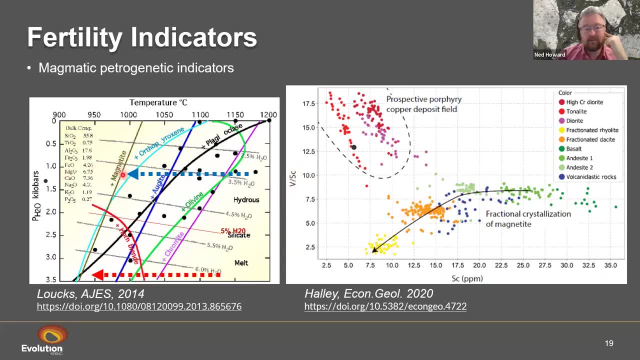 ratio also decreasing as we're crystallizing magnetite. however, if we've got wet magmas we would expect to see that ratio increase. so the intrusion that'll be prospective for for porphyry deposits that are relatively wet we would expect to plot up here so we can discriminate those two. 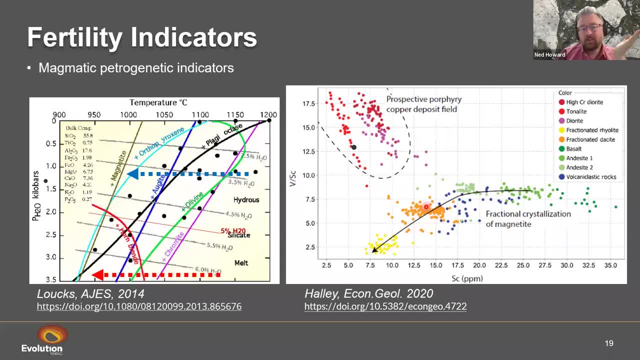 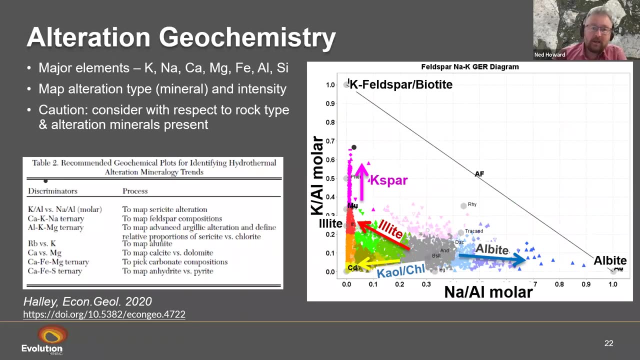 out. but but this is all really going back to the geochemistry of reflecting, reflecting geological processes that are that are happening within those magnets. alteration geochemistry is another thing that we can can do, so here we're more looking at the major elements, so potassium, sodium, calcium, magnesium, iron, those kind of things which will tend to move around. 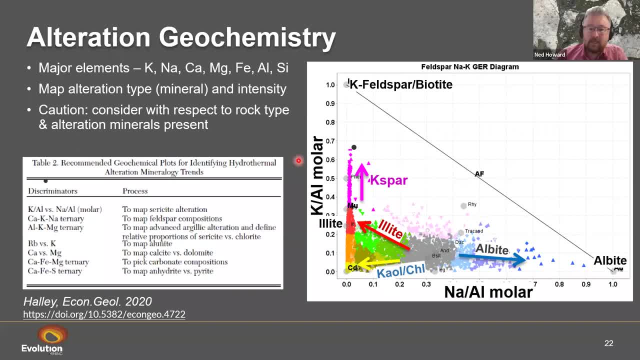 hosted in our, in our major silicate minerals, and so with looking at the geochemistry in various ratios we're able to map out different alteration related processes that might be happening in these rocks and also the intensity or the extent to which they've happened. so this is a common diagram here. 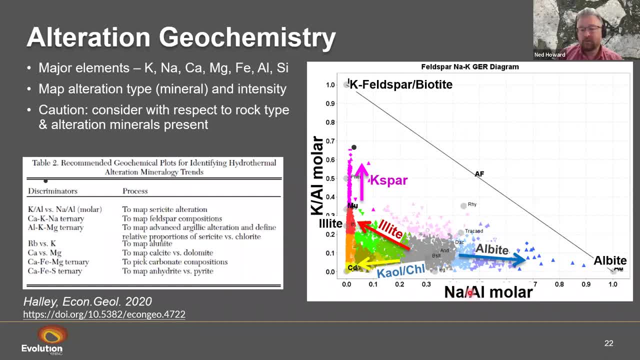 that we can use, which is plotting the molar ratio of sodium over aluminium against the molar ratio of potassium over aluminium and so on. this we can plot where pure minerals would plot if we, if we had just those pure minerals analyzed. so albite will plot over here because it's got, there's no. 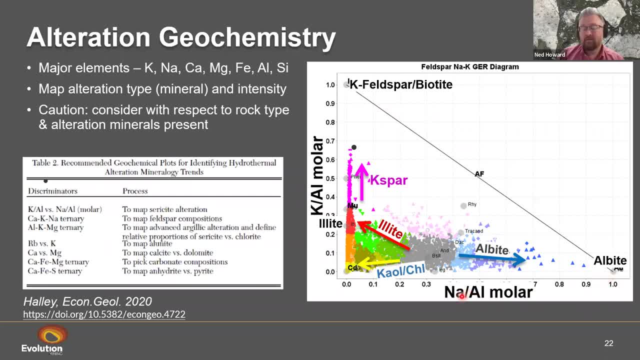 potassium in it and there's one, there's one atom of Lion from that nutrient here and the another can be observed on the trucs at mine under 30% Atmosphere. one atom of sort of sodium for every one atom of aluminium within within the chemical formula case bar or the by. we'll pull it up here. 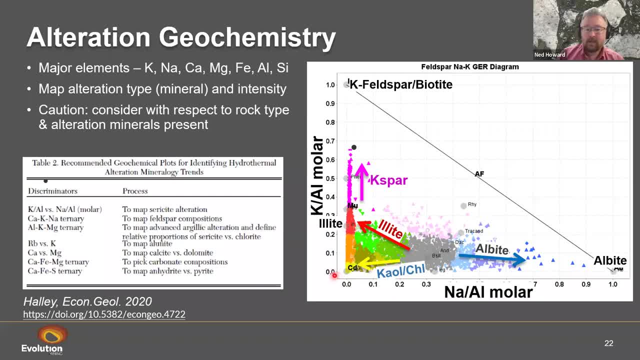 Atmosphere. one atom of sodium for every one at of sodium for every one atm of aluminium within within the chemical formula case bar, or it will pull it up here- muscovite would point around .33. you're like a little bit lower and down at. 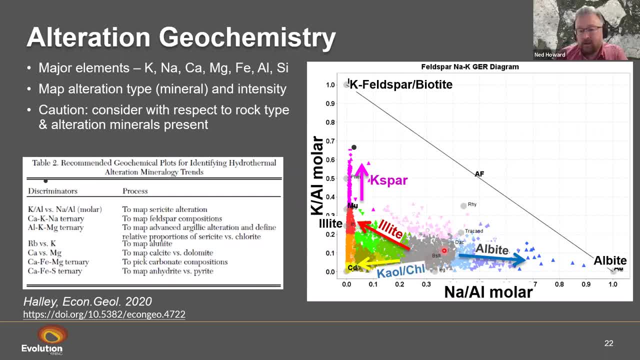 00 we expected See things that could be either be cable or call right. 00 we expected See things that could be either be L tonight board or chloride. 00 we expected See things that could be either B СоEven I bow. they'll pull it up in further in this direction. 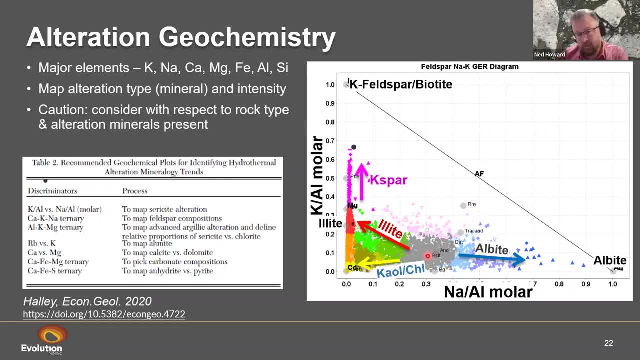 But the trends we see associated with different alteration assemblages will usually travel in different directions, And so if we're seeing albite, related albite alteration, we'll see samples move out in this direction towards the albite node. If we're seeing illite or white mica or sericide alteration, 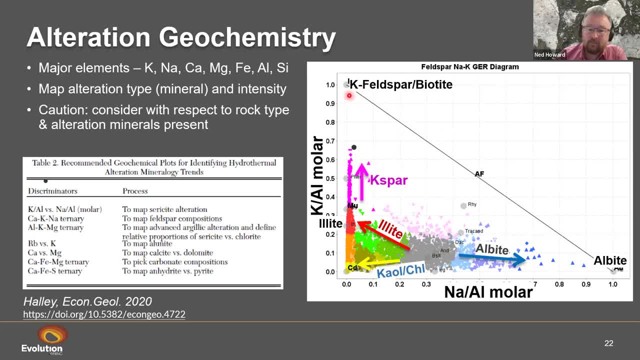 we'll tend to see things move out in this direction, case bar move up this way, or if it's kaolinite in weathering or agilic alteration or chloride, we might see it move down here towards the origin. So the important thing to remember with this: 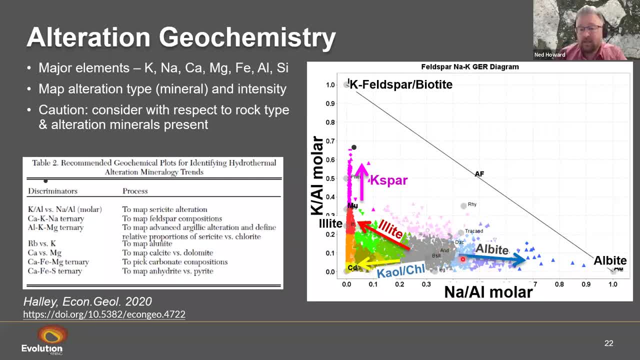 is that we're talking about Bockrock chemistry here, that the distance something moves is proportional to the relative alteration intensity of that type, And also that we talk about this in respect to minerals, but it does not mean that those minerals cannot be present in rocks that are plotting here. 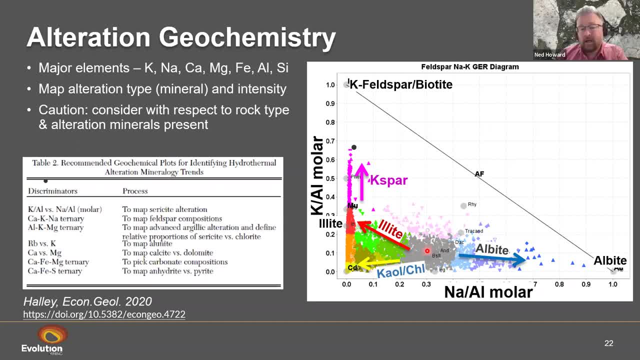 So you can have sericide alteration in a rock that's still plotting with the same overall potassium over aluminium ratio. But what it means is that that has been isochemical on a whole rock basis, So it's only used the potassium in the rock to create that sericide. 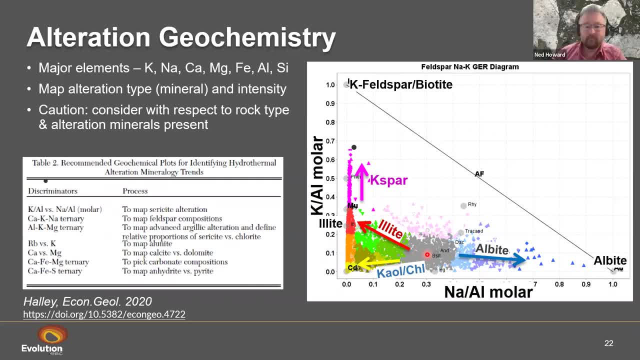 It hasn't added any extra to do that. So these can have sericide, chloride, albite, whatever in them, these rocks here, but it's only using those components that were originally in the rock rather than adding them, which is what you're doing. 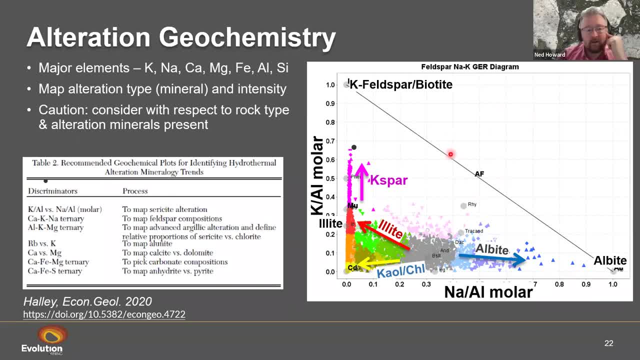 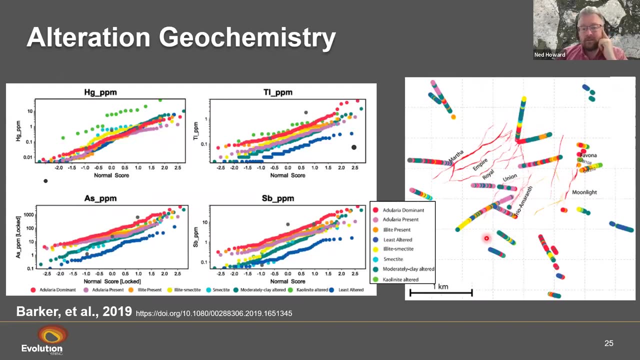 as you travel along these lines, And so there's a whole bunch of other diagrams like this that we can use to map out different hydrothermal alteration zones around our projects. So to show an example of that, this is from the Waihi deposit, which is a low sulfidation. 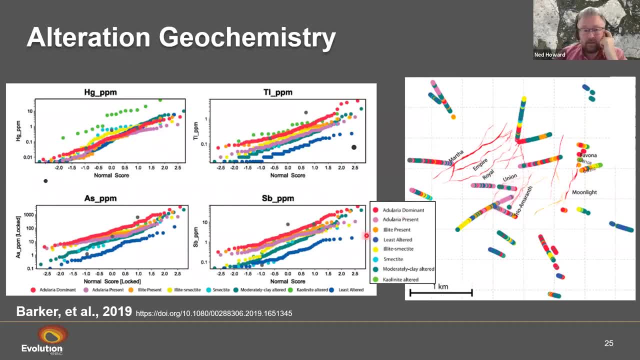 epithermal deposit in New Zealand, And so you know we've done a classification. the Barker et al have done a classification here on the basis of those different groups. So where we're seeing agile area, alteration, illite, illite, smectite, smectite, kaolinite. 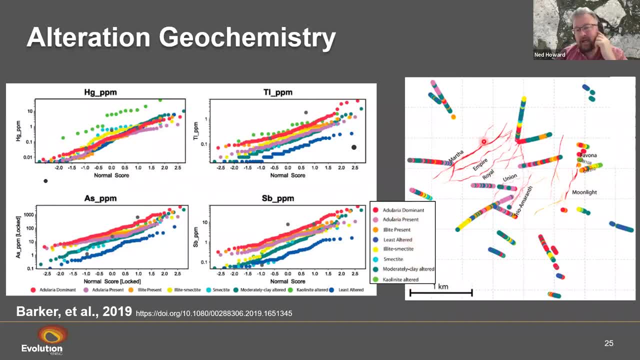 at least altered in the blue, And you can see here this is just plotting that over the presence of veining within that high sulfidation, that low sulf epithermal deposit, And you can see so where you're seeing a lot of agile area in a zone that's defined. 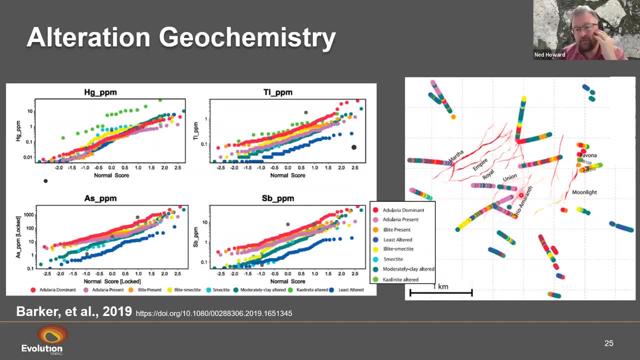 around this area of increased vein density through there. The other thing we can do with this is look at the relationship between what we're mapping out. So we're looking at the relationship between what we're mapping out and what we're mapping out In those major major mineral alteration mineral groups and see what the relationships 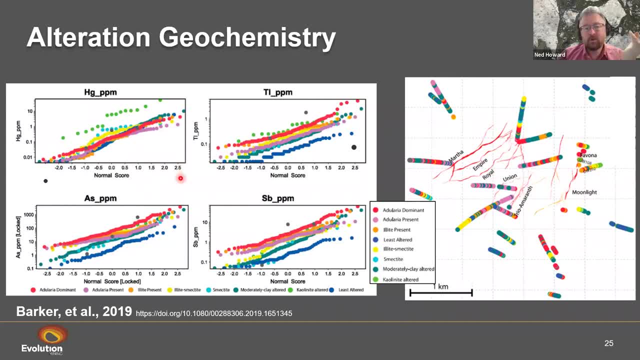 are with our pathfinder elements as well, Because usually we'll often we'll see similar, similar patterns between those minerals, which gives us a more robust understanding of the architecture of the hydrothermal system. So in here we're seeing you know where we've got the agile area dominant. we're seeing 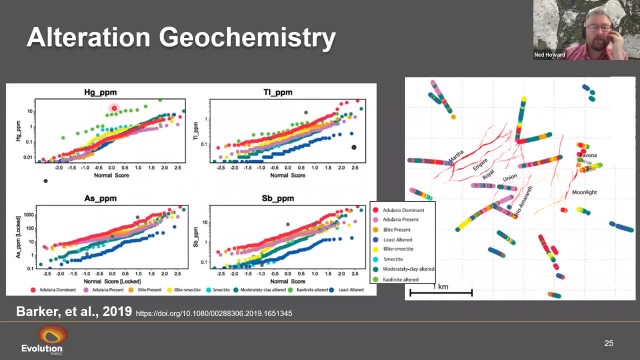 more arsenic, more antimony, more thallium, but, interestingly so, where we've got the caolinite alteration, which is probably steam heated alteration sitting at the very top nearest, near near paleo surface environment, is where we're seeing elevated mercury, which 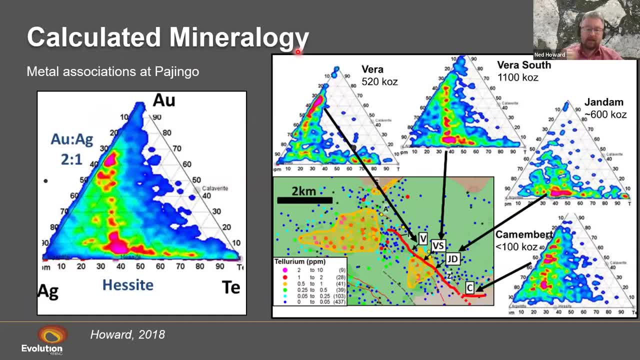 is what we expect there. Another thing we can do is look at mapping out differences in the in the mineralogy throughout deposits. So this can be useful for a demanding point of view once you're getting into more advanced projects and need to start thinking about the properties of the ore- whether it's hard. 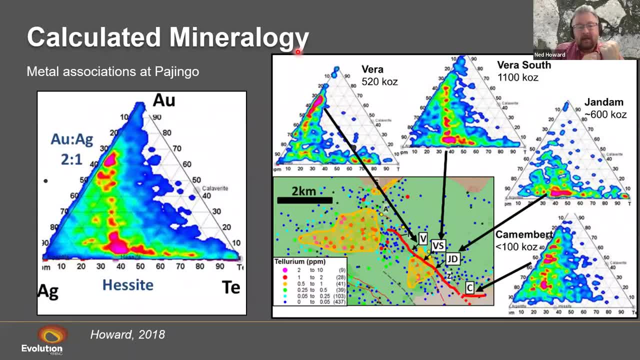 or soft, it's going to produce a lot of clay or not, and what is associated with the gold and whether it's going to be relatively easy or hard to to leach that gold out of the rock during processing. So this is just an example from Pajingo, where we've got a ternary diagram just from samples. 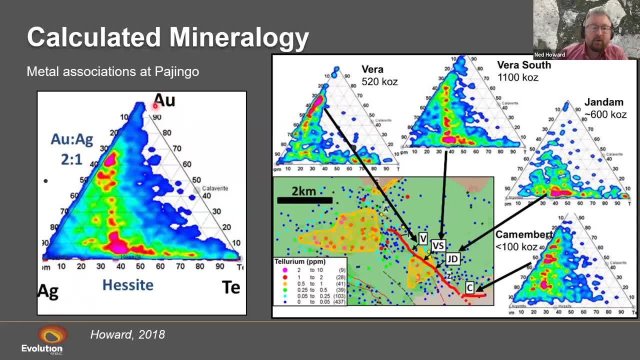 of mineralized veins And we can plot, Do a point, density, plot in the ternary diagram from gold to tellurium, to silver, and we can see different associations that are sitting in there. So we see, you know, there's a bit of a cluster here that would be defining electrum association. 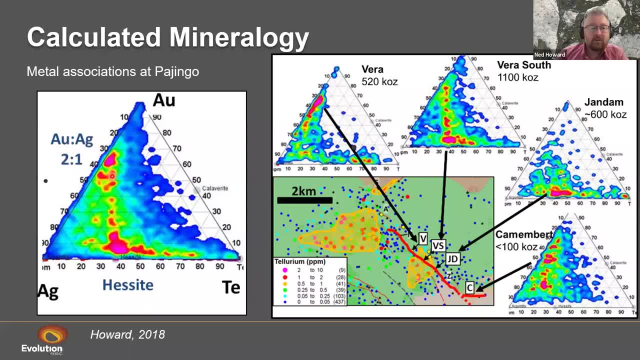 around with, you know, two to one, gold to silver, But then also there's a node here sitting around hessite. So where we're still, we're seeing gold, but it's in association with that hessite, telluride. 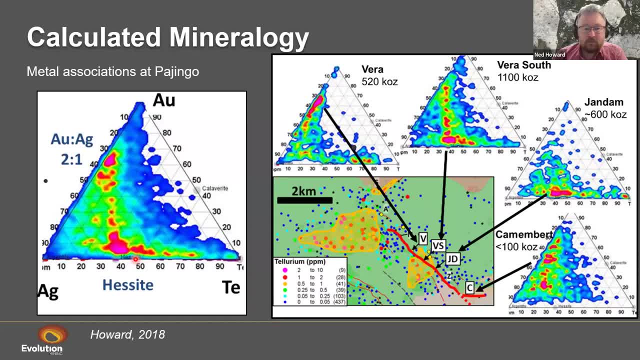 which can Increase your reagent consumption And potentially decrease your recovery. And interestingly here, So we can look through these different or zones along through the Pajingo low sulfidation epithermal vein system and see that we're seeing changing associations through those deposits. 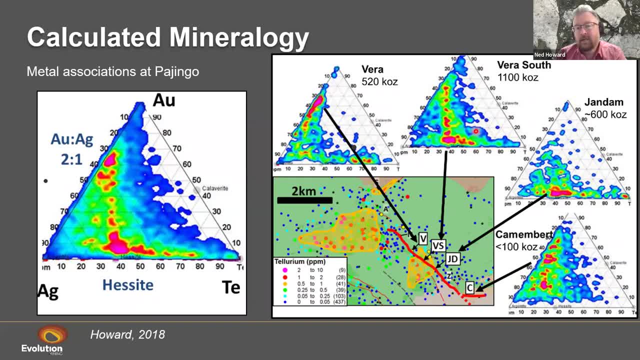 So potentially so, from Vera. we're seeing more electrum dominated in Vera South and and Jandam. We're seeing Things plotting around that, that hessite node, more. So there we, you know, we're seeing Changes in those mental logical associations that could be associated with with different properties, when we're when we're processing those different 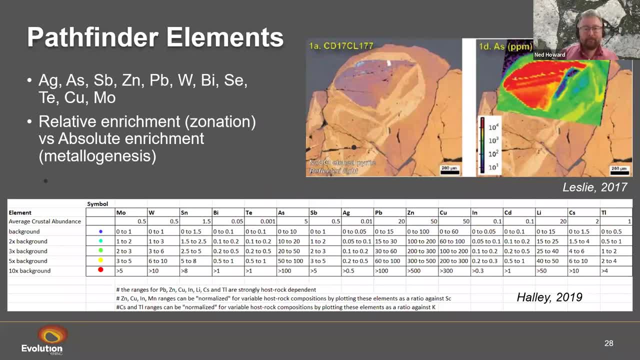 Or So. to jump now to to Pathfinder elements: There's a pretty typical suite of that 10 or 11 elements there that always like to To Analyze for, And so what we're usually looking for with Pathfinder elements and need to be thinking about is 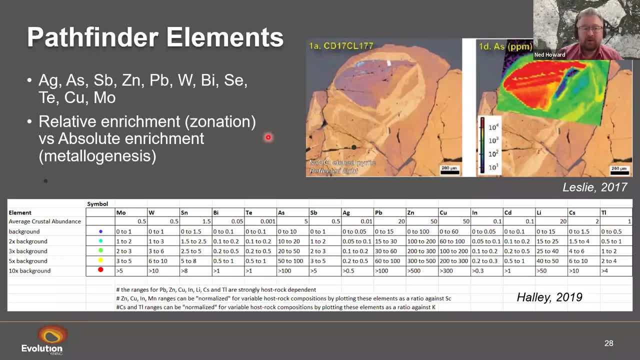 Is what's controlling their distribution? what kind of geological processes? and so most of these elements are, a lot of them, governed by how they substitute into pyrite. so thankfully, pirates are pretty common mineral. it's usually Compared to a lot of other minerals that might be hosting trace elements is 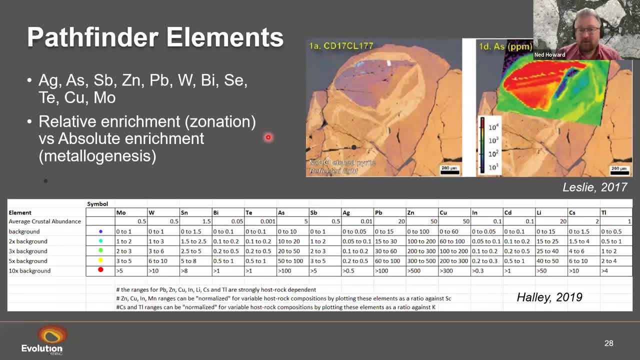 relatively homogeneously distributed through a rock mass, Depending on the style of deposit you've got, which means that we can pick up these changes in concentrations of these different elements relatively easily. And so the two things that usually have the biggest impact on on the substitution into pirate of these, these elements is usually temperature and also pH. 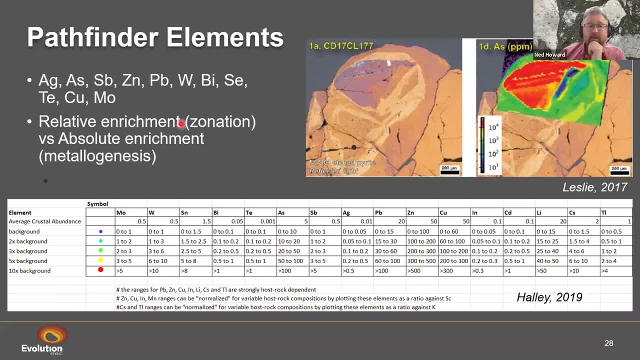 is another important one. One thing to remember with Pathfinder elements, though, as well, is that so he's from from Scott Halley on his website again- is some some good. you know baseline ranges to use for for plotting different Pathfinder elements, but every mineral system is a little bit different, so start with these, and then you may find that you need to modify things. 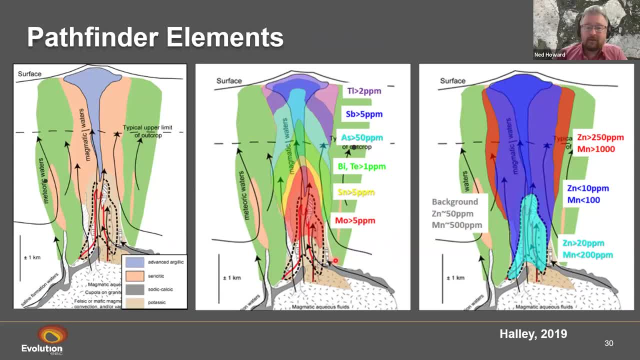 So, So, So, to look at the typical patterns that we, that we often say, This is an example from a, from a porphyry system where we've got porphyry couple molly style for mineralization through here, forming relatively deep and around prophecies, offer, offer, bath lift below. 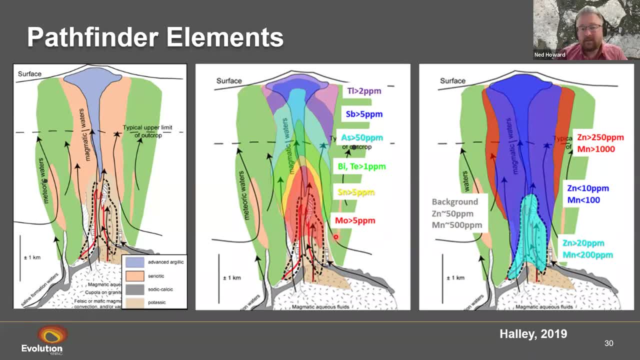 As those fluids travel up through the system. we tend to see, as our nation, from elements that Substitute into- Excuse me, form higher temperature sulfides or substituting to pirate a relatively hot temperatures, through to those that tend to substitute in at relatively low temperatures. so going from things like molly 10 business to Lurian, through the things like arsenic and timid and salient. so this is defining a temperature. 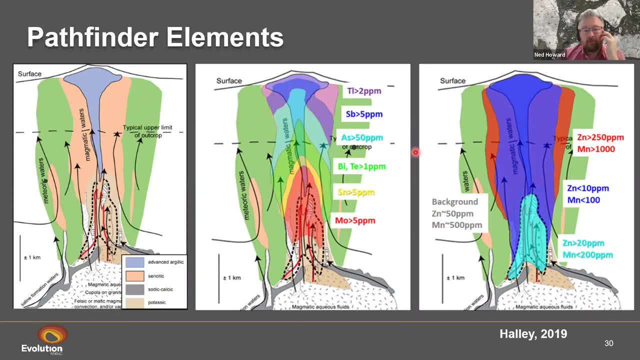 Gradient and we often see Particularly in the portrait epithymal environment these temperature-based zonation patterns within their pathfinder elements. An example of where we're seeing pH-controlled patterns is around the behaviour of things like zinc and manganese within those kind of systems. So we tend to see in the middle of the system through here and where. 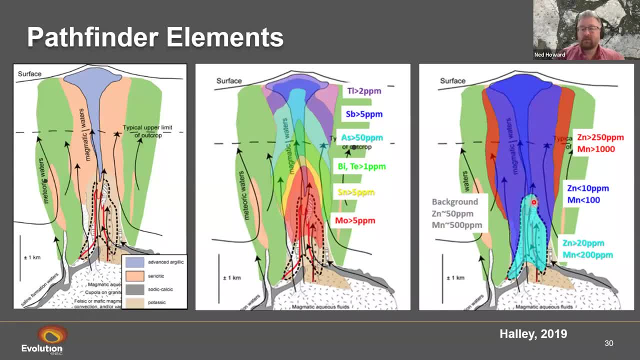 we're dealing with. as we get cooling we get more acid fluids within which manganese and zinc are relatively mobile, so they stay in solution, they don't get precipitated out. But then near the edges of that system where we tend to encounter pH gradients, where we might be seeing mixing between 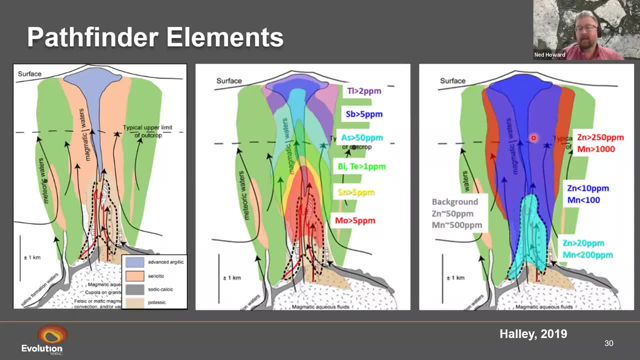 these increasingly acidic, magmatic-sourced fluids versus circulating higher pH groundwaters And so on. those pH boundaries where we're going from lower pH to high pH is where we'll start seeing higher concentrations of things like zinc and manganese being precipitated out. That may be into pyrite or maybe into other things like sometimes you can get quite a lot into. 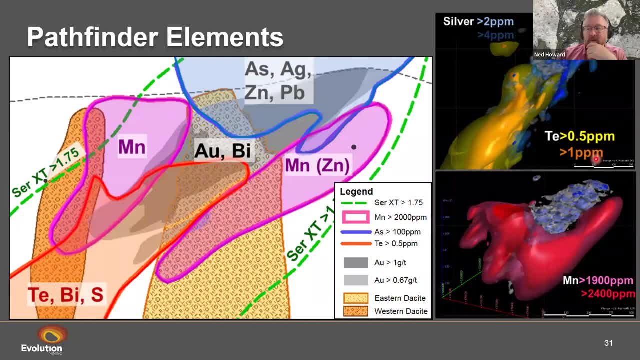 chloride or carbonates as well. So another example of that here, looking at these pathfinder elements, where we're seeing that this is the Mount Rawdon, which is a kind of epizonal intrusion-related gold deposit in Queensland. So the ore body is shaded out here in grey and we can see that it's associated with this kind of. 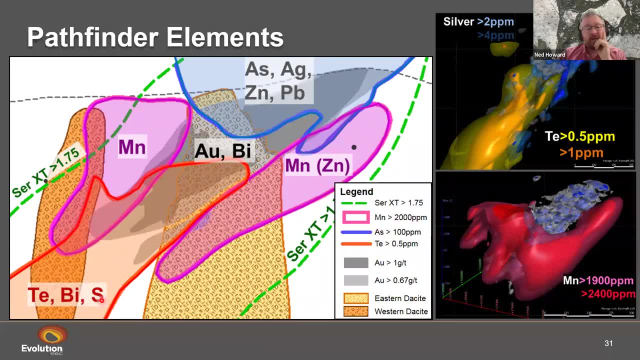 central plume of bismuth and elevated bismuth tellurium and sulphur Gold's most closely associated with bismuth, which is something we often see in these intrusion-related systems. but then it's zoning up to get increasing concentrations of arsenic, silver, lead and zinc. 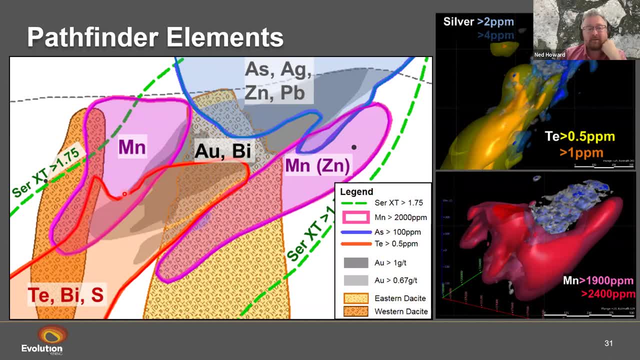 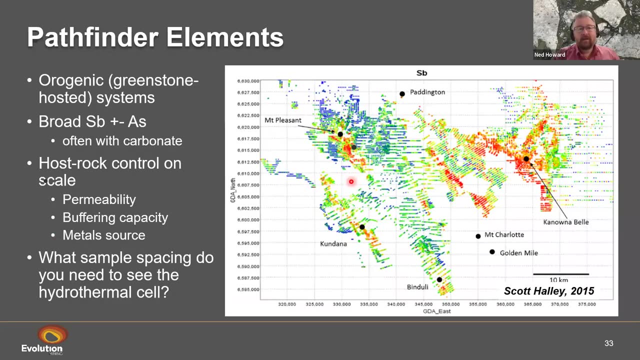 Up the top and we see these halos of elevated manganese and a bit of zinc around the outsides as well, where we're seeing these sitting in chloride and carbonates associated with that pH gradient, Pathfinder element footprints. particularly when we're talking about orogenic styles, there's 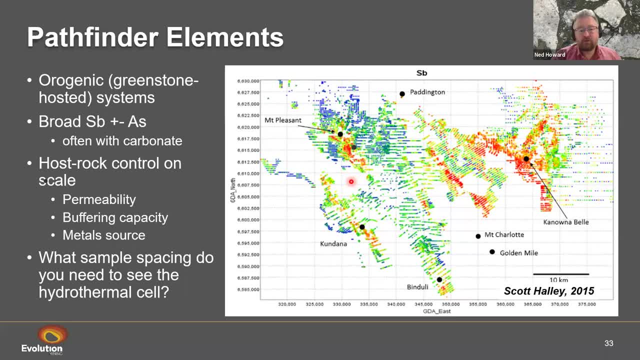 I guess often people will emphasise how restricted the alteration halos can be around orogenic deposits, and that can be true in terms of their proximal alteration, but usually these things are sitting within hydrothermal cells that have much larger footprints. So this is an example here of a data set from the Kalgoorlie area, where you 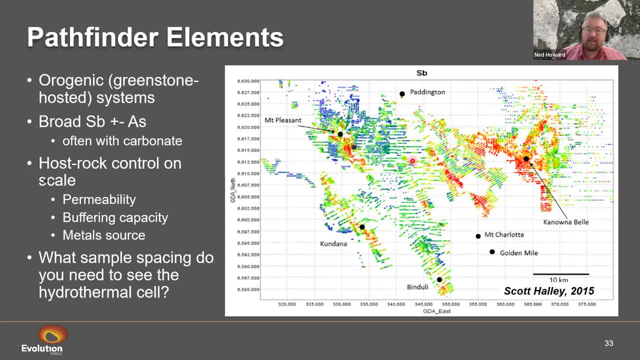 can see. so everything that's red here is where we've got antimony above about three or four ppm, and so all the big gold deposits and gold deposits can be found within that. So the gold deposits can camps through here, sit within plumes of of antimony that are also usually where you're. 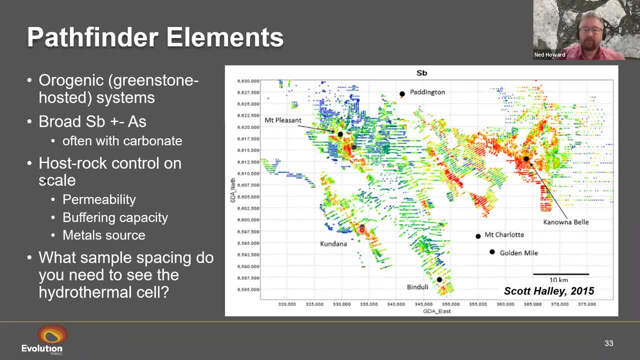 seeing broad zones of of carbonate alteration as well. you'll see there here, though, that there's there's quite a range in the in the size of those. there's a there's a host rock control to that where we see this in mafic rocks. they tend to be more restricted relative to the size of the camp. 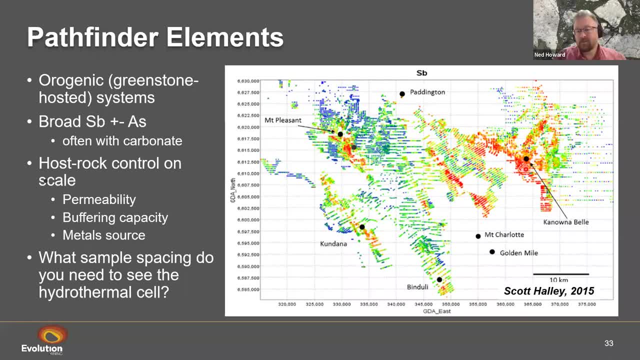 the size of the gold deposits compared to things like canada bell, which is, you know, seven million ounces but has this huge halo around it, whereas at kandana, where we've got about the same gold endowment but a more restricted yet still large halo around that. so when you're interpreting these, 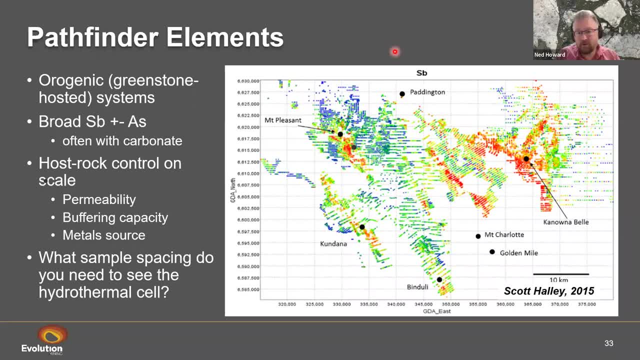 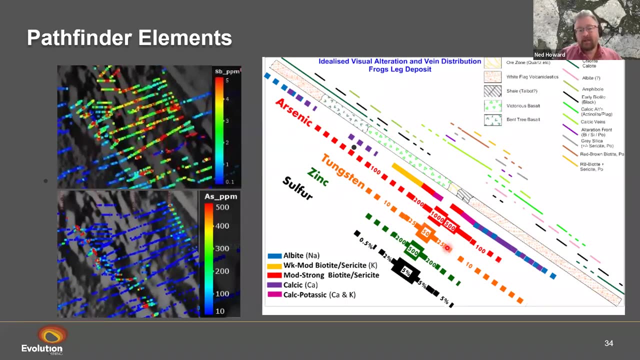 kind of patterns. you need to be thinking about controls of host rock permeability, the buffering capacity of the host rock. if we zoom in on the kandana type deposits, you know. the other thing we can use pathfinders for is is different pathfinders often will have. 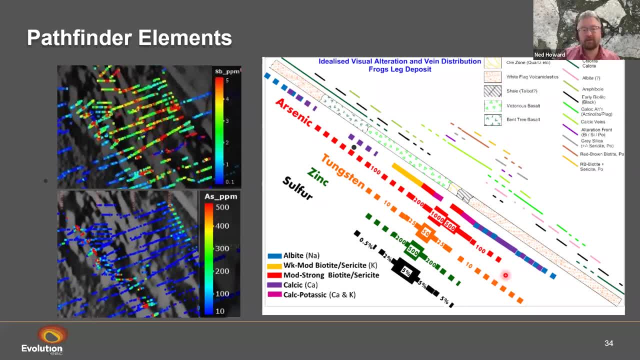 different scales of footprints or different associations around around deposits. so just talking about the importance of of antimony, which we can see over here, this is a zoom in here where we're seeing, you know, quite a broad area that's. that's bringing us into into the kind of camp 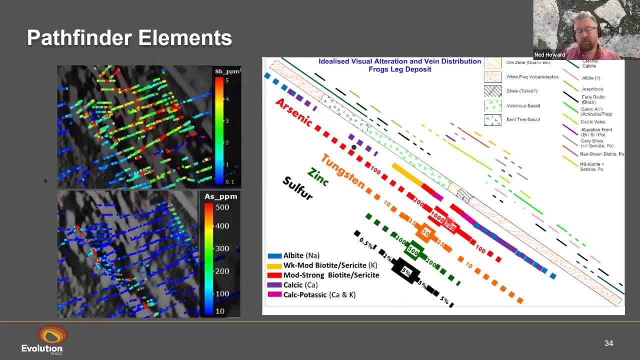 scale there. but when we're trying to start look towards, looking at zoning, towards um, we're towards a particular deposit. uh, we might be looking at different indicators um. so in this case you know it looks. uh, arsenic, tungsten, zinc and sulfur are more useful for kind of proximal. 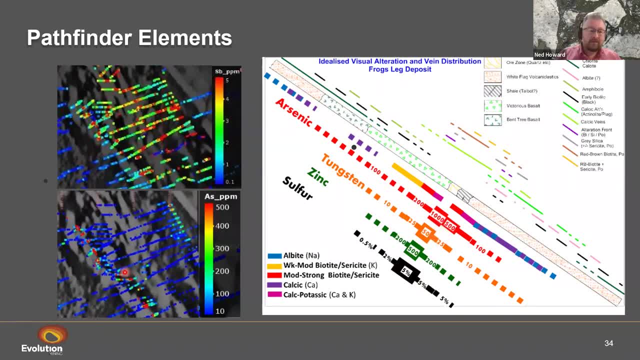 vein related um elements. so we're kind of seeing that here we've got this nice big uh halo in the in the antimony, but then when we look at the arsenic, in this case over the frog's leg deposit, we're seeing quite a tight relationship there along the all hosting structure. regolith is another really important thing to to be. 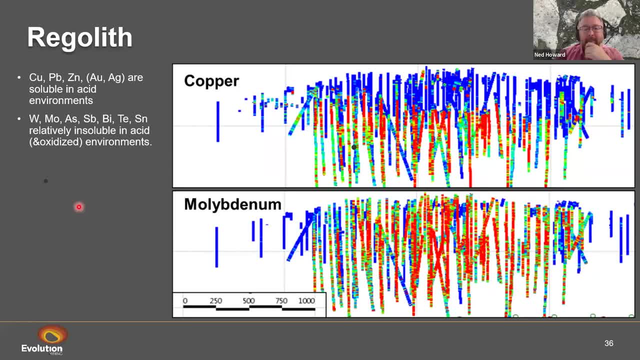 thinking about as well. so, um, and the the behavior of different elements in this. so a lot of you- if you're from Western Australia, we're familiar with you- know the deep weathering environments that we get over there, where a lot of elements- those that are low valence state- will tend to be. 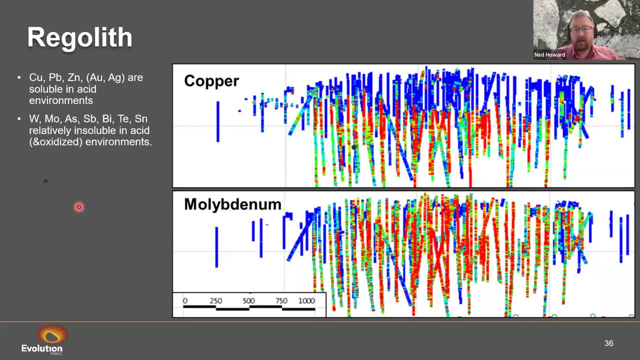 um leached out of um, out of the the upper parts of the weathering environment, as we would see for for copper in this example, um, where we're seeing this, this leaching out of the upper part of the weathering profile. then we've got a super gene enrichment Horizon where that's being 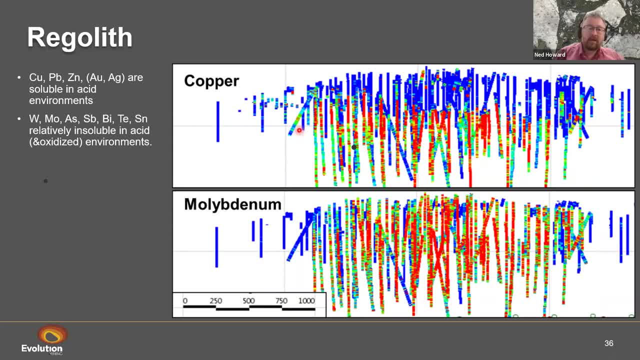 re-precipitated, and then the bedrock concentrations underneath that. so things like copper, lead and zinc will tend to behave in that way, but some of our other Pathfinders, things like tungsten moly and lorium um will that are that are higher valence state, will tend to be less soluble in the oxidized 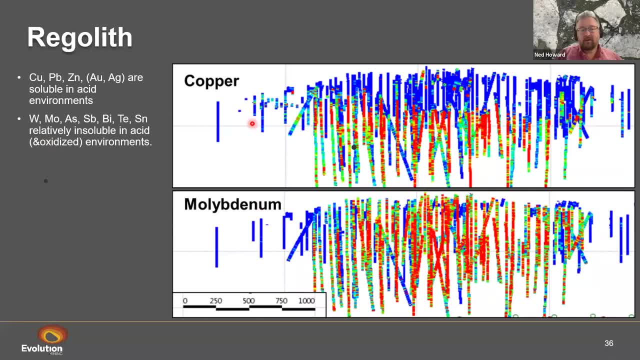 acidic ground waters that are that are leaching this copper out. so this is, you know, the the same: porphyry, copper, gold deposit, copper, moly deposit. you can see that the copper has been leached out of that surface environment, whereas the moly's been retained. so if you're doing surface sampling, 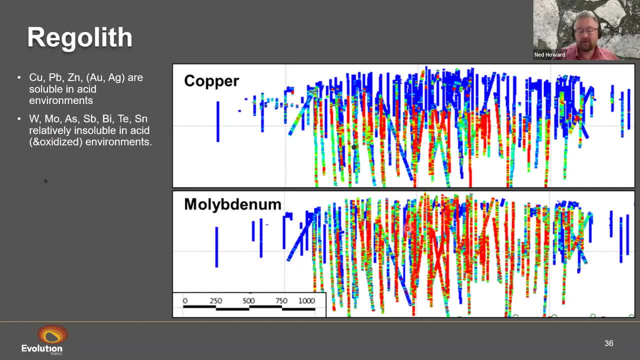 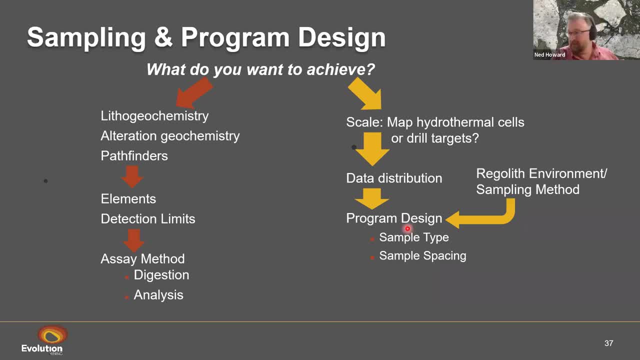 uh, and looking to define a nullies. you know you need to to understand the different element behavior in the context of the regolith there. um, I've only I've run a little bit over time, so I'll just skip through some of this a bit more quickly. but just to talk a little bit about sampling and program. 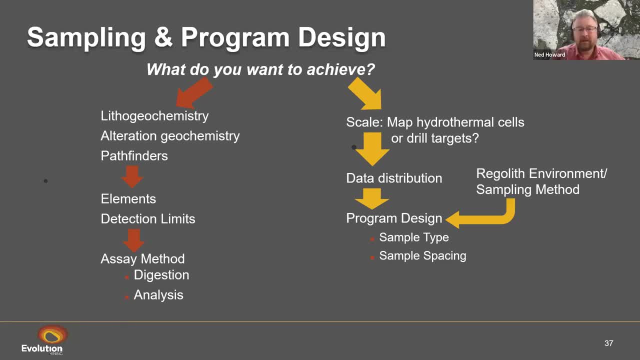 design. so it's- it's really important when you're looking at using geochemistry for some of the purposes we've discussed, that you you need to think about two things really, and that's: what kind of analysis method are you going to use? and that's going to define what you're able to do with that data. and the other thing you need to. 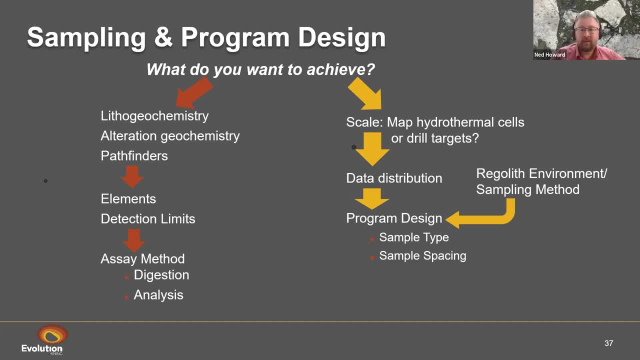 think about is program design. so what scale do I need to either map out the hydrothermal cells that I'm if- if that's what I'm trying to do, or if I'm trying to map drill targets? what's the? what's the scale that they occur at and the scale of the anomalies I expect to see associated with? 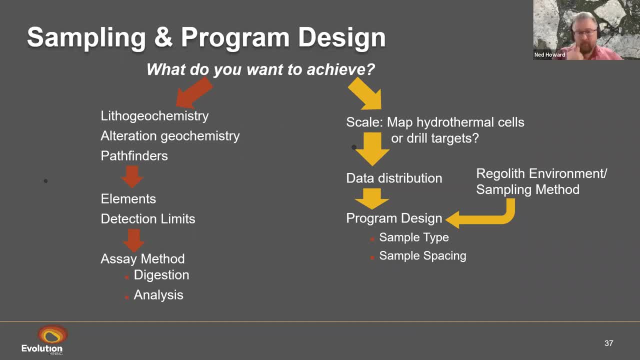 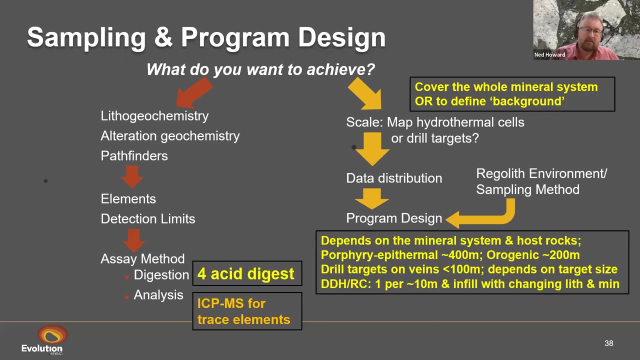 it to define what your sample spacing is going to be, whether that's downhole or in soils or end of hole. grab that kind of thing. you also obviously need to be thinking about your um, your regolith environment and sampling methodology as well. so for all of this, I'd say that in most cases a four acid digest analysis at a good lab there is. 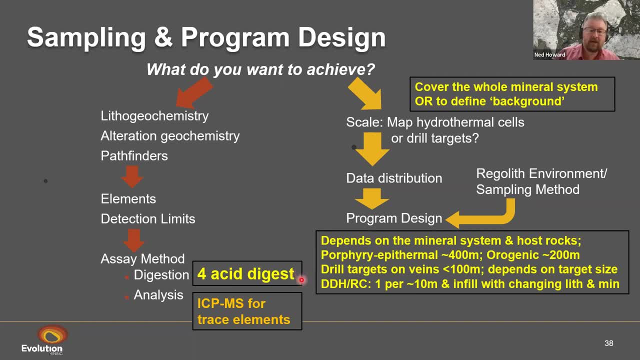 quite some variability between labs in the. in the quality analysis you get but four acid digest um within ICP-N MS finish for your trace elements is usually the best way to go. if you do- if you want to do, you know any of this kind of stuff- you can cut down your analysis suite but usually it's only a. 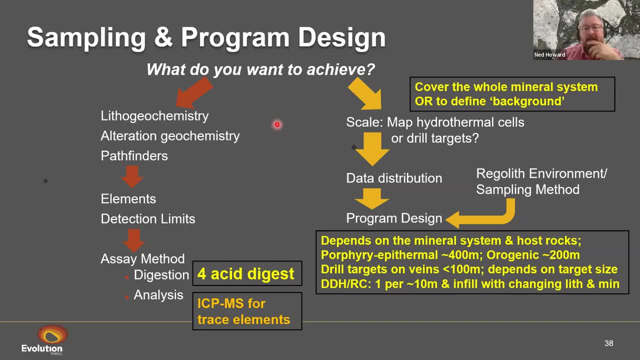 relatively incremental cost saving that that limits what you're able to do with the suite in terms of the spatial distribution of the sampling. you can your- your you're looking at um- try and cover the whole of the mineral system or at least to define background relative to what you're looking for. so if you're trying to define zones for targeted 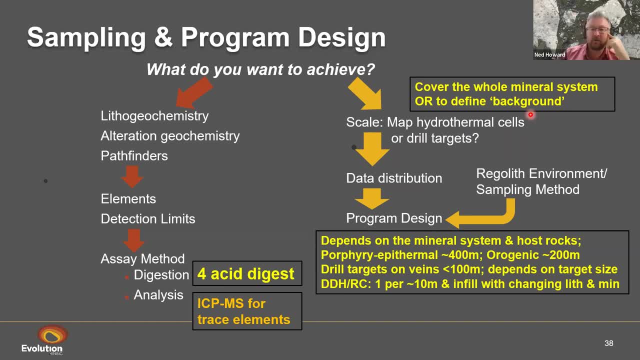 drilling on a on a particular structure, you need to make sure you're covering- you know- a significant length of that so you can define what's high, low, what's background. with project program design usually you can get away. if you're trying to map out mineral systems, um, initially. 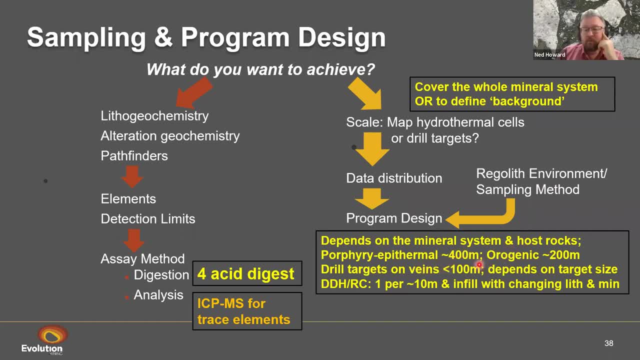 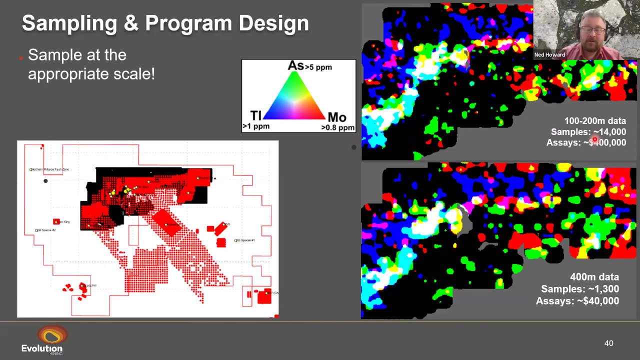 um, you can get away with some quite broad spacing, but it does depend on the geological environment that you're in, and if you're trying to define drill hole targets, usually closer spacing is is better and more important. um, to touch on that with an example, uh, this is one from the the 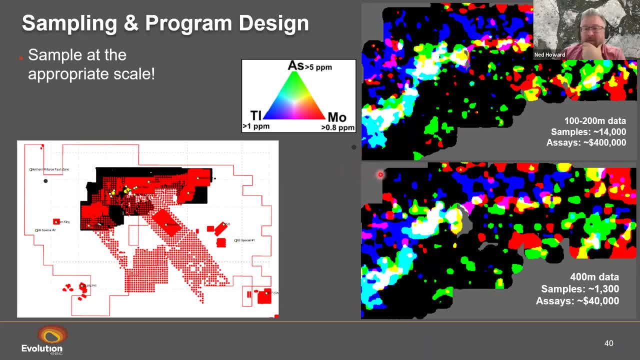 Mount Carlton deposit um where I worked some time ago. these two diagrams here are called RGB images um percentile cutoffs, where we're looking at three different trace elements that have different associations, proximal through to through the distal, so we can map out um where we think we are proximal. 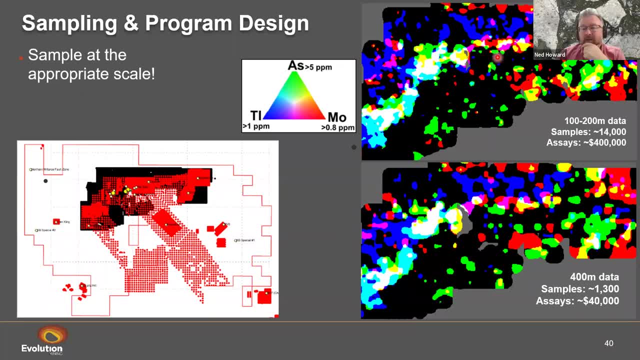 distal, more highly or less abroaded in the in the mineral system. you can see both these images are pretty much the same. so we're mapping out things um pretty pretty much the same between these two things. so this is the original data set, which is mainly 100 to 200 meter sampling um spaced samples. 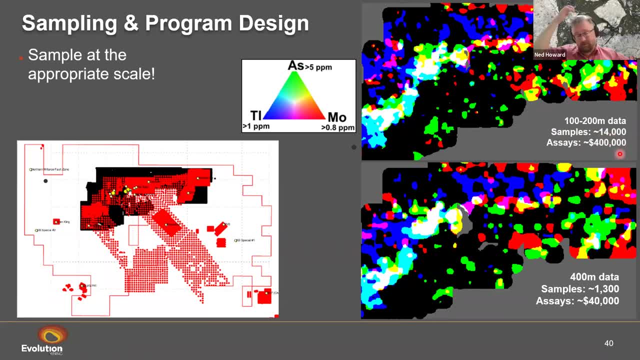 that's 14 000 samples at an assay cost of four hundred thousand dollars. we could get pretty much the same map in terms of zoning into where we want to do some more concentrated follow-up work, with 400 meter spaced sampling, which would mean one-tenth the number of 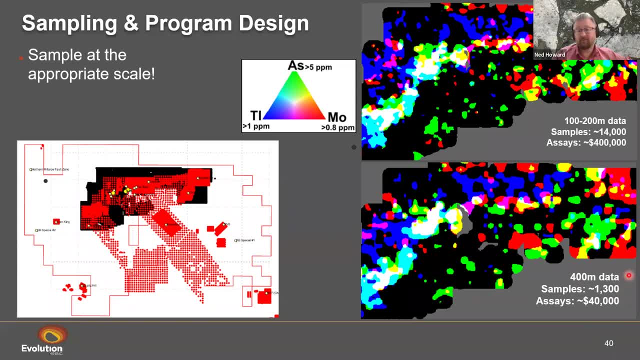 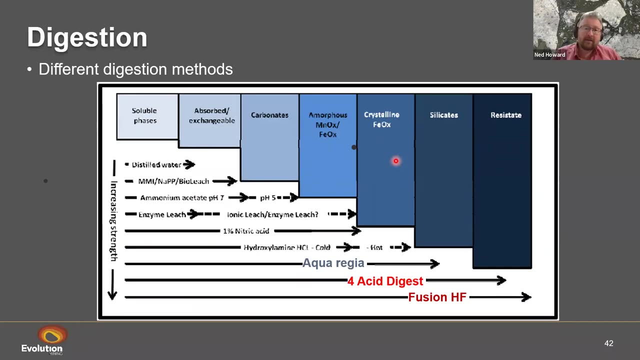 samples and the cost and, significantly, the amount of time, um, that it would take to do this. so you really want to be thinking about what is the scale. I need to be able to define the patterns I'm looking for, um, when we're looking at analysis, digestion is is a really important thing to consider. 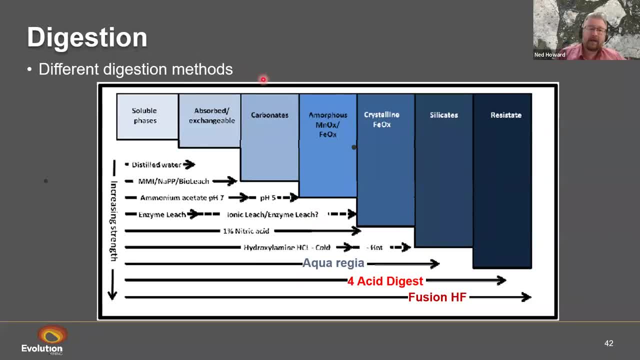 um, so usually when we're samples are being analyzed, they're being digested into a solution so that that can then be be run through a machine like an icpms or an icp or an oes. but the type of digestion you use, which is basically mixing up powdered sample in a 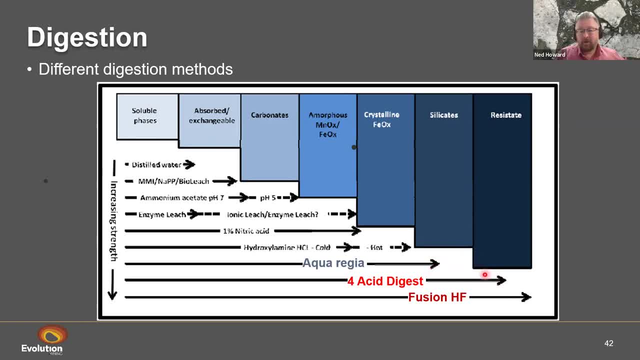 um in a concoction of acids, the, the type of concoction basically, will determine how much of that sample and which minerals you're going to dissolve, and so that's a a really important consideration because if you want to look at things like um, your trace elements for doing, 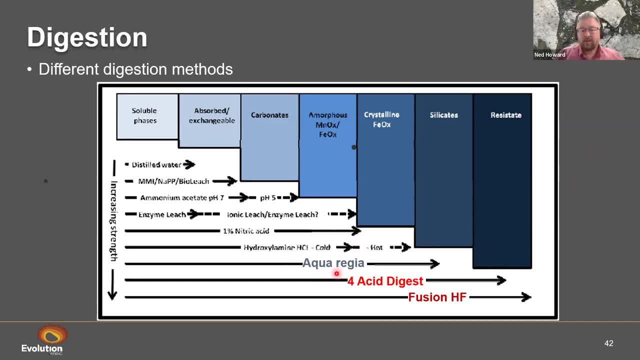 with the geochemistry um, you're not going to dissolve all of those elements with aqua regia. you'll get almost all of them with four acid digest if it's done at a good lap. you'll get pretty much all of them if you do a fusion and then a digest after that. but there are there are things that you'll you'll miss. 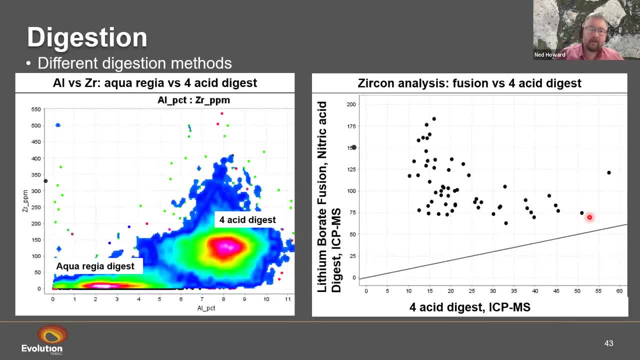 out on if you do a fusion digest. so if we have a look at that, we can see the difference here between an aqua region digest where we're just not dissolving um our either our silicates or our resistant minerals like zircon, versus four acid digest. 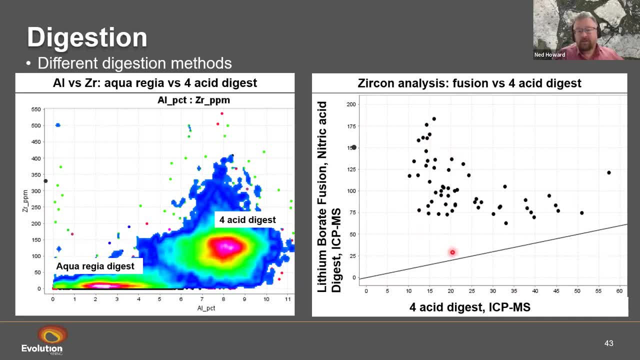 where we, where we are um with some four acid digests, and particularly where you've got zircon, um well, zirconium sitting in zircon rather than other minerals, we'll tend to see that the lithium borate fusion, which is fusing the sample to glass before that you try and dissolve. 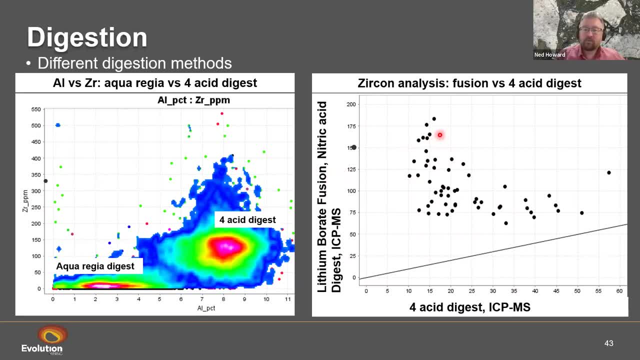 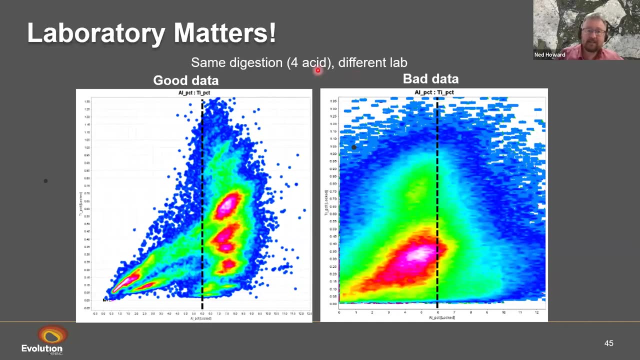 it. so you're overcoming those mineralogical controls and so we'll see really poor uh fusion in some cases. um, with the four acid digest relative to the lithium borate, but there's a really big lab control on that. so this is the example here comparing two different labs. so 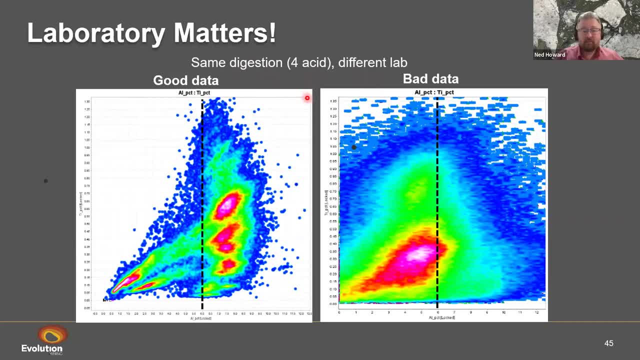 this is a four acid digest- essentially the same process on the face of it. this is at a at a good lab who's got good practices and done things properly, and where we're dissolving everything into solution before we run the final analysis and you can see how much you can discriminate here in these different rock units. this is from. 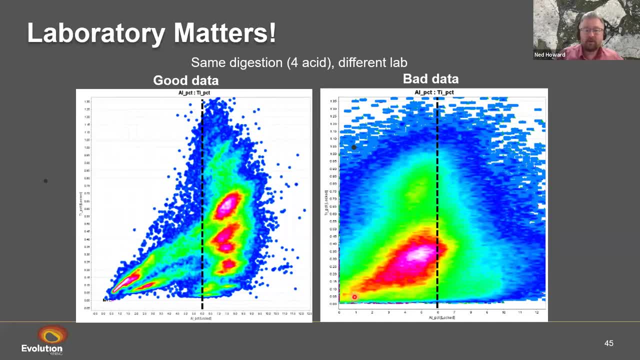 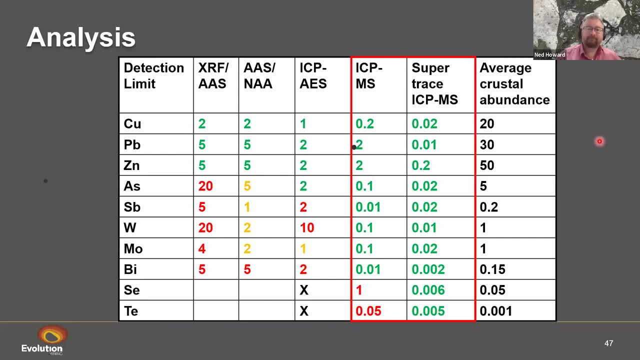 the same area where we're seeing the same rock units, and all we've got is this overall messy kind of cloud. so it does matter where you get your samples analyzed. when we're looking at the, at the finish we use uh. it's really important to consider this both in terms of the the elements. 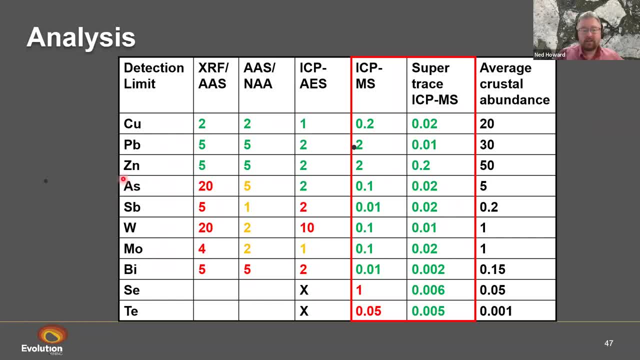 that we can analyze for and the detection limits, particularly with our Pathfinder elements, um analyses that are done historically or or at the moment by things like AES or OES analysis methods, you don't get the detection limits that you need to fully resolve anomalies in these elements compared to their typical crustal background. so if we take bismuth, for instance, 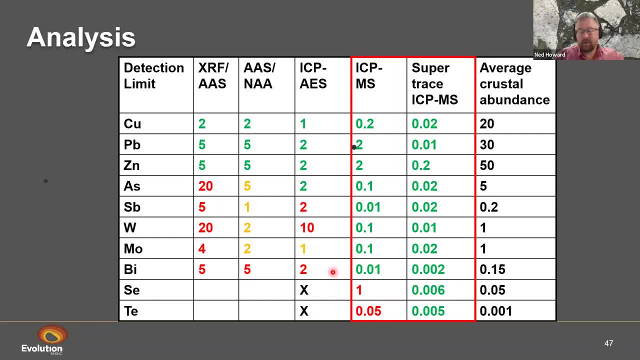 um. so if you get um uh four acid digest within icp, OES um finish, you might get a detection limit of bismuth. but the average crustal abundance of business is about 0.1 to 0.2 ppm, so you're not.